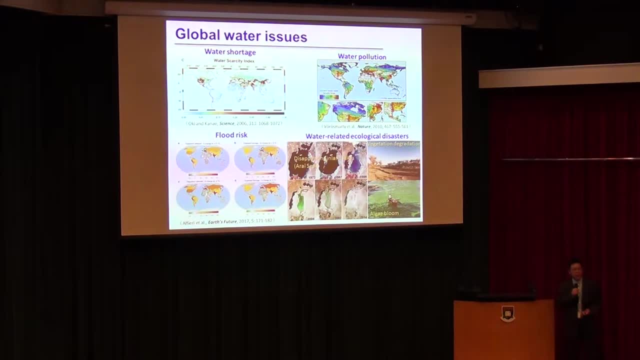 So the background is: the entire world is facing severe water issues, many challenges. water challenges, For example, water shortage, water pollution, flood risk and many water-related ecological disasters, such as disappearing inland lake, like vegetation degradation and algae blooms. 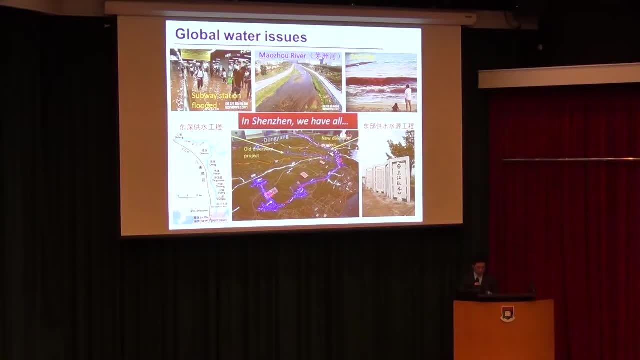 So these water issues actually are not far away from us In the city I'm living, in Shenzhen. actually, we have all these problems. For example, the subway stations are frequently flooded during big storms, And Shenzhen has several very highly polluted rivers like Maozhouhe. 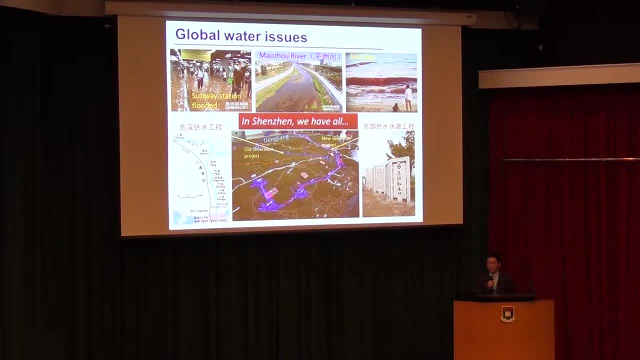 And also in the near shore area, we have red tide due to algae blooms. And in Shenzhen, although we have a lot of rain every year, but the water supply is mainly from outside of the city. For example, we have two water diversion projects. 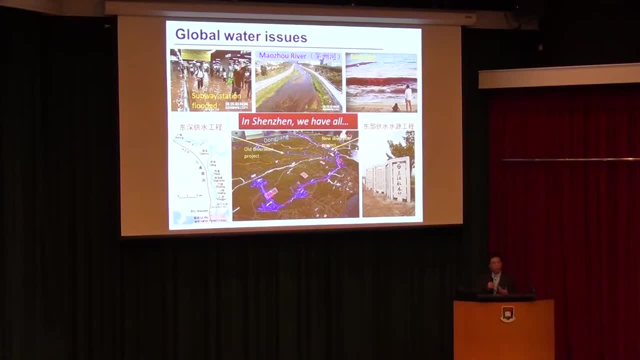 One was built like half a century ago which also provides water to Hong Kong. That's the old diversion project, And about early this century We had another diversion project to supply water from Dongjiang to Shenzhen city. So even in wet areas Shenzhen is still in great shortage of water resources. 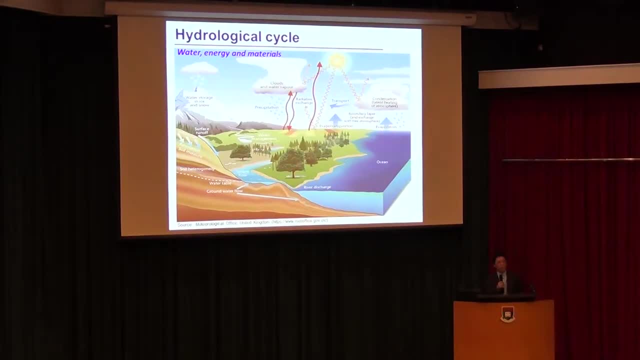 So, to address all these water issues, it's fundamental to understand the hydrological cycle of the earth. So, okay, So let me spend a couple of minutes to explain the hydrological cycle. So, as you may know, the water can evaporate from the ocean and from the land into the atmosphere. 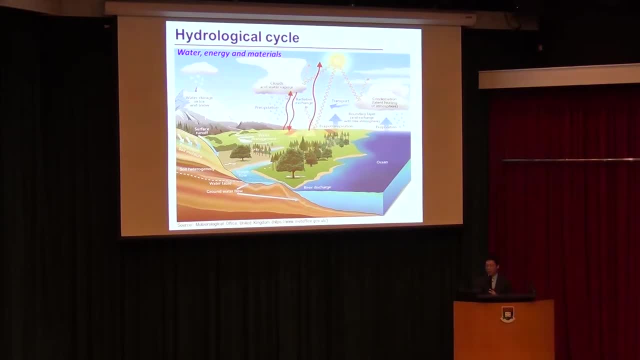 Then it can become a cloud And it can produce precipitation in terms of snow or rainfall. So when the precipitation reaches land, it creates surface runoff Or it infiltrates into soil all the way down to a saturated air zone we call the groundwater. 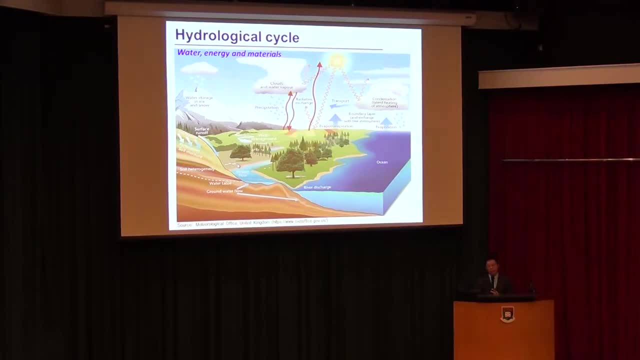 And both the surface water and groundwater can flow from high land to low land and eventually come back to the ocean. So that's a very short description of hydrological cycle. So hydrological cycle is actually coupled with energy cycles of the earth. 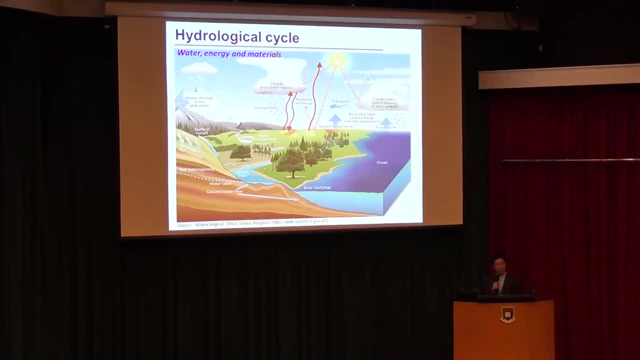 And also it's the driving forces for the circles of many other materials like carbon nutrients. So basically it's critical to the earth. So the importance of hydrological cycle to the earth is just like the importance of blood circulation to humans. 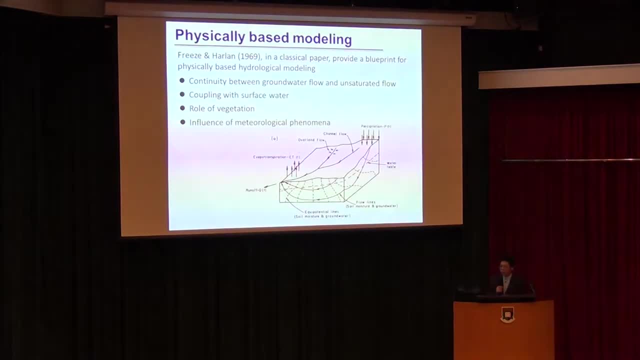 So we need to understand the hydrological cycle And also to quantitatively describe it. In 1969, Fritz and Haaland wrote a classic paper which provides a blueprint for physically based hydrological modeling. So actually the current ongoing hydrological modeling is still following this blueprint. 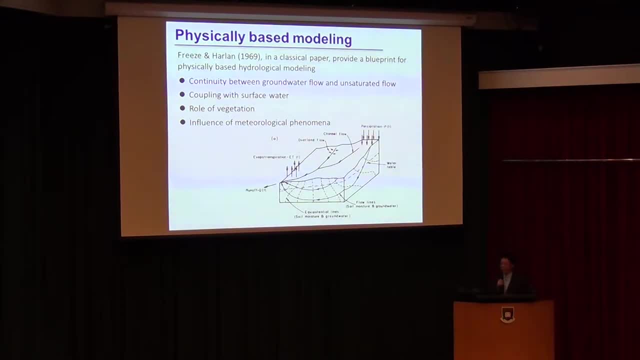 So this blueprint emphasizes the following things: First is the continuity between groundwater flow and unsaturated flow, And the second is coupling with surface water with groundwater. And the third is to emphasize the role of vegetation on the hydrological cycle. And the fourth is to consider the influence of meteorological phenomena. 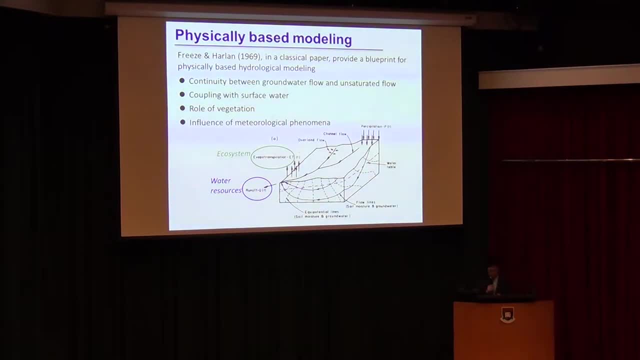 So I just want to say that, I just want to emphasize. So the modeling mainly address two variables. The first is the runoff, That is, the flow out of the watershed. So why this is important for the modeling? Because it's a measure of the available water resources to human beings. 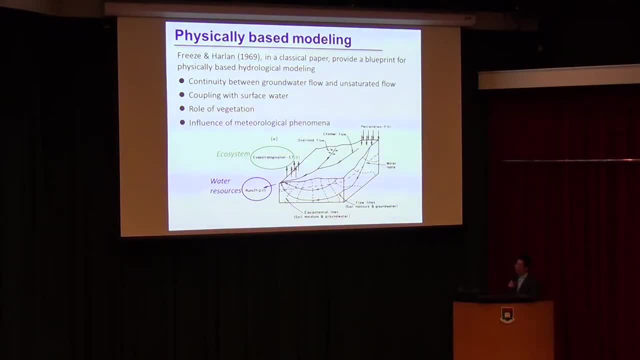 And the second variable key to the modeling is the evapotranspiration, Including evaporation and transpiration. Why this ET is important? Because it reflects the activity strength of the ecosystems on the earth. So basically, these are two variables most concerned by hydrological modeling. 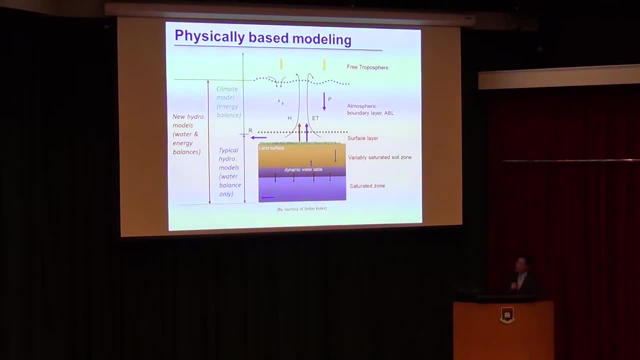 So physically based modeling. So this figure just brings a column from the subsurface into the atom, From the atmosphere. And, as we can see from this figure, Typical hydrological models actually address this portion, That is, from the saturated zone. 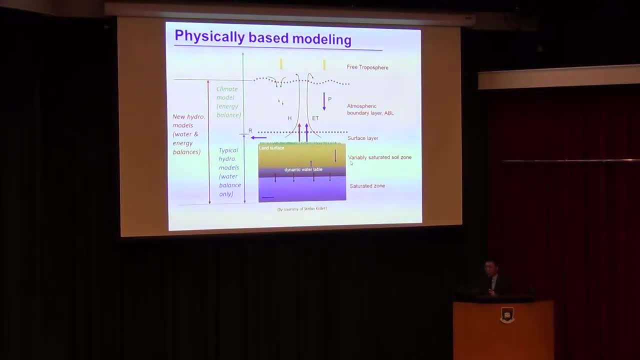 The zone saturated with water, The groundwater, The variably saturated soil zone And the surface layer Which includes vegetation. So that's the zone that typical hydrological model address And the typical hydrological model Consider water balance From here above into the atmosphere. 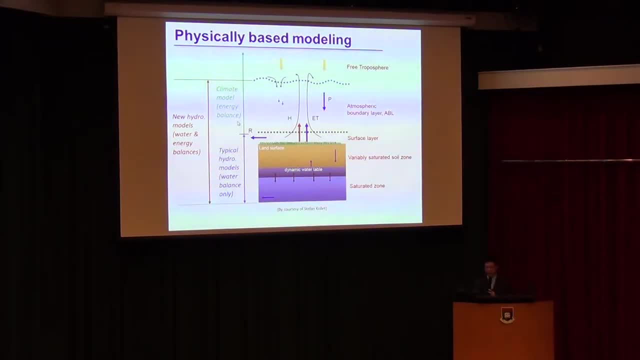 That's the job of climate model, Which mainly consider energy balance. So now our society is developing the new generation of hydrological models Which include the atmospheric boundary layers into the modeling frame. So this range Is what is the new generation of models concerned about. 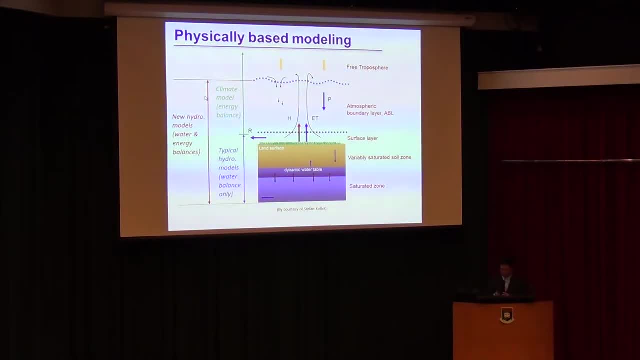 Okay, So this reflects the idea To modeling from the subsurface into the atmosphere, So by considering both water and energy balances. So I apologize that this slide is the only slide that have differential equations In my presentation, So, but I won't explain all these differential equations. 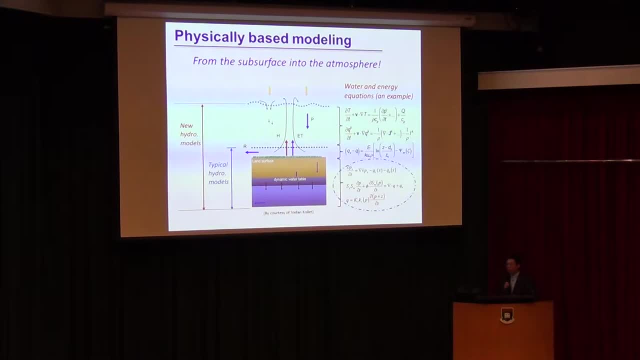 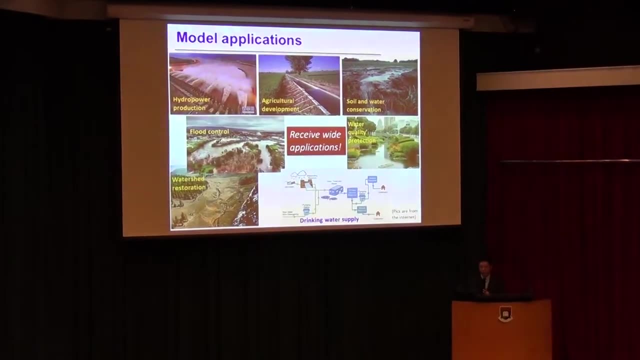 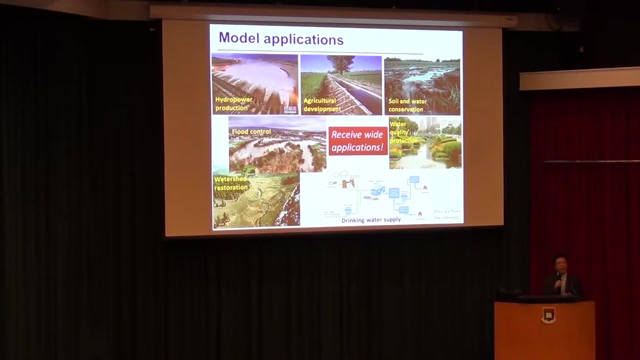 So this just give you some concept of what kind of hydrological model I'm talking about. Okay, So, although the physically based model is still under development Following the blueprint, It has been widely used in water resources management, For example. 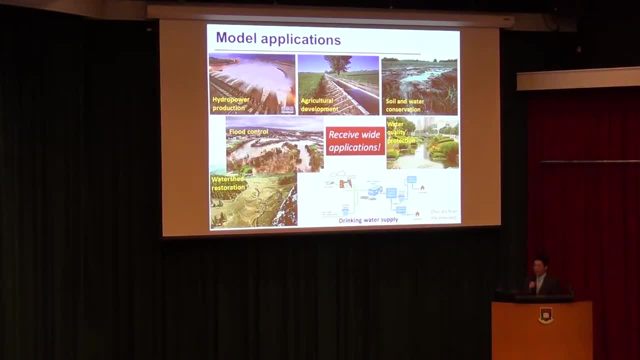 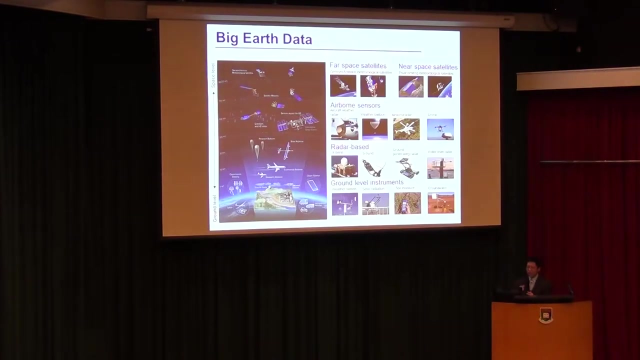 To support hydropower production decisions, To support agriculture development decisions For soil and water conservation, Flood control, Water quality protection And watershed restoration. Just mention a few. So the physically based models have already been widely used. So let's look at the other side. 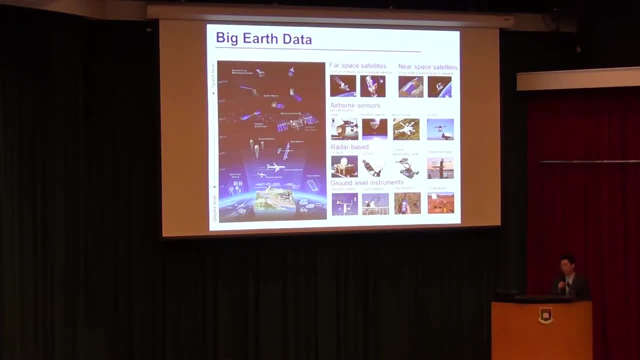 Data. So in our community We are talking about big earth data. So this year A new Chinese journal titled big earth data is coming to. It's just being brought up. So what big earth data? Because we have all sorts of sensors devices. 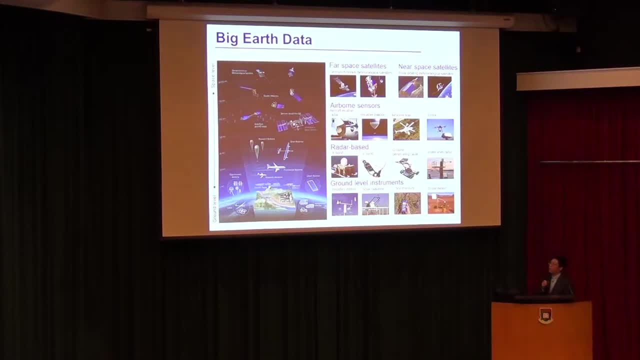 To observe the status of earth From many different aspects, From the ground level Into the space level. For example, We have fast space satellites, Near space satellites. We have airborne sensors On different platforms, Like aircraft, Weather balloon, Helicopter, drone. 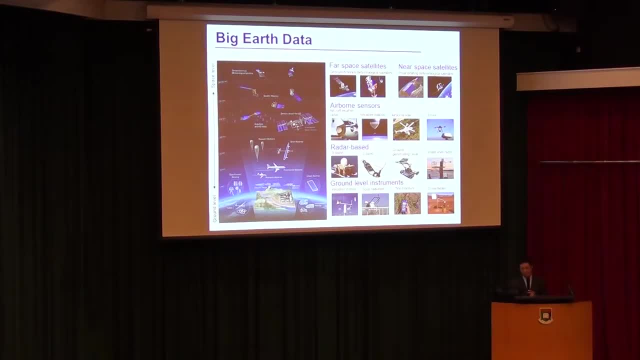 Also at the ground. We have all sorts of radar To measure different variables Of the earth. Also, we have very traditional Or classic ground level instruments Like meteorology stations. We have solar radiation observation devices And other measurements. 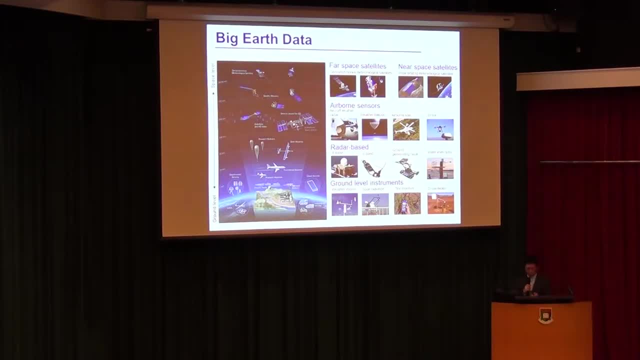 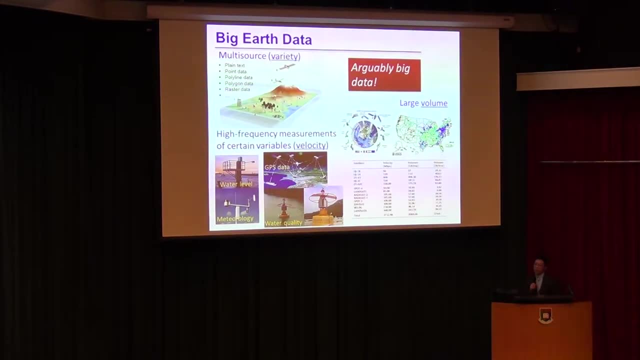 Okay, So we have all sorts of data Related to the earth That we call big earth data. So big earth is arguably big data, Because I know in other fields People have different definitions About big data. So some don't think. 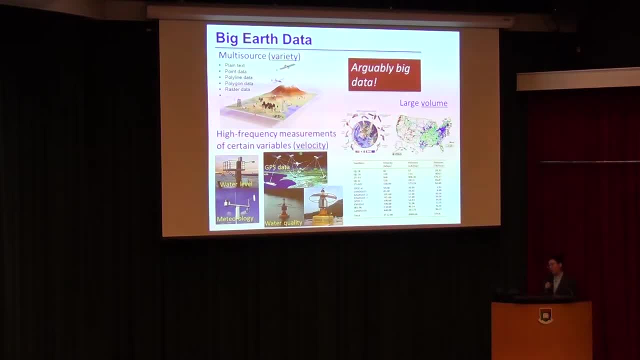 The data I mentioned Are really big data, So I say it's arguably big data. For example, It has at least three features: Variety, Because all those sensors Collect multi-source data And some data are in plain text, Some data are in point data. 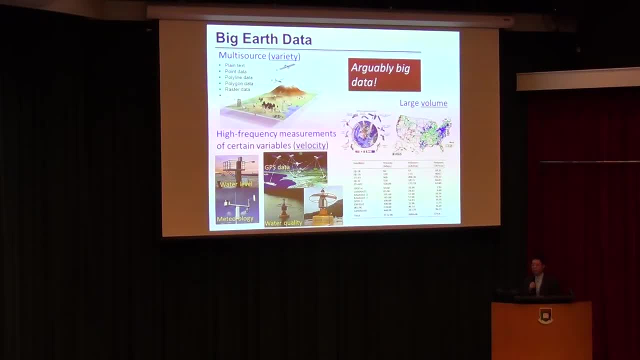 Also we have point line Polygon data, Rust data, So multi-source, With significant variety, Also the large volume. So we know the. So the data need to reach a PB level So we can call it big data. 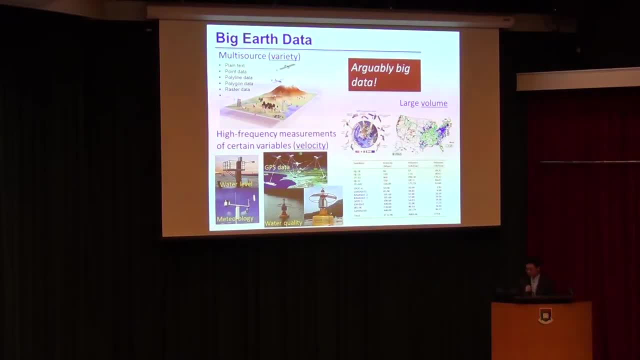 So with all these satellite data, Actually the big earth is reaching that level. Okay, Also velocity: We have some high frequency measurements In our area, Like we can have real time Water level monitoring And we have high frequency measurements. 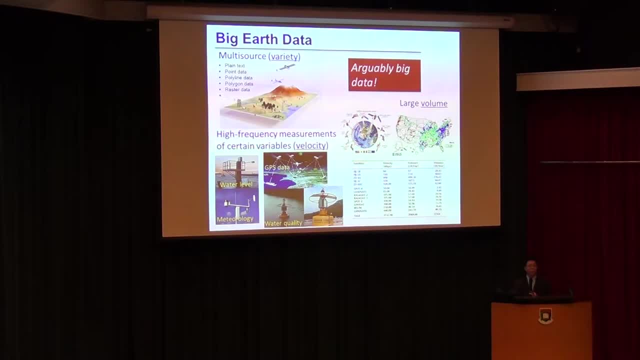 Of meteorology variables. Of course, the GPS data Is the most typical data With high velocity, Because any time We are receiving a lot of GPS data, Okay, And also like in area of water quality monitoring, So we have monitoring system. 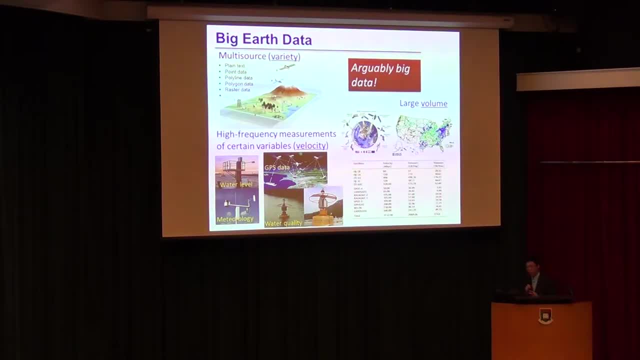 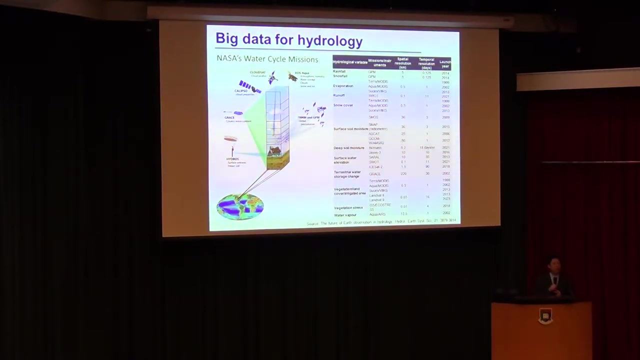 Like give you a very high frequency measurement Of the water quality. So arguably, We have high velocity of the data transfer From all sorts of sensors. Okay, So for hydrology? So the big data Mainly from satellites? 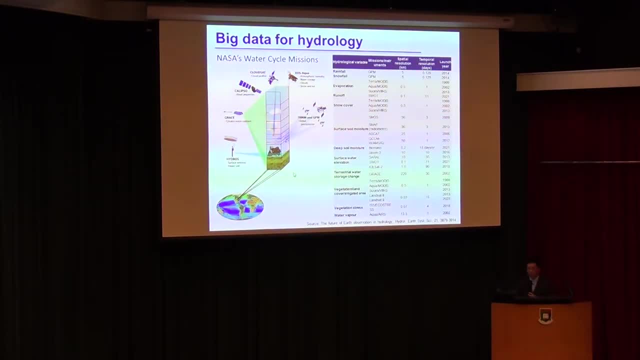 For example, This picture shows NASA's water cycle mission. So it launched many satellites Carrying different kind of sensors. So different sensor can measure different aspects Of the hydrological cycle. For example. This, like GRACE, Is the most well-known satellite. 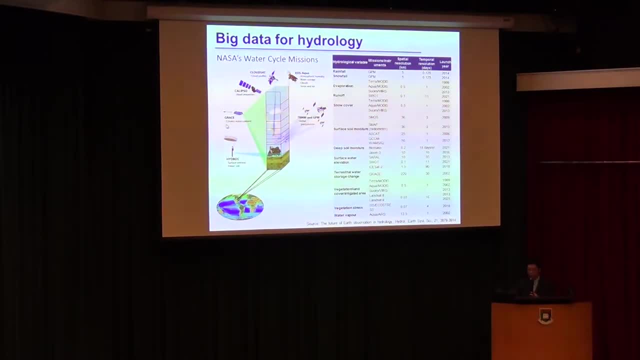 To provide the water information. So it measures the column water content Of the earth And if it has preserved some change Of the water storage, It mainly reflects the change Of the water stored in soil And the ground water. Okay, 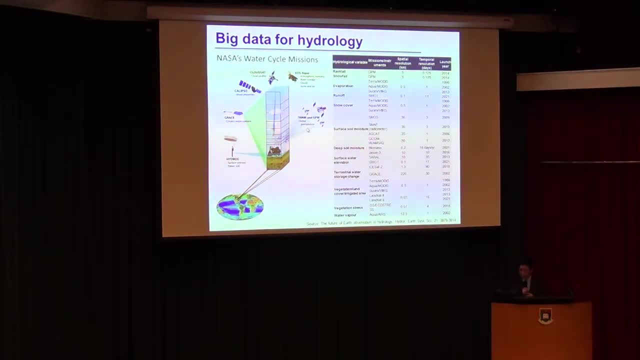 Also, trim and the GPM Are the most used Satellite data For global precipitation estimation. Okay, So this table also Gives you a list Of all the hydrological, All the main satellites That provide the measurements Of major hydrological variables. 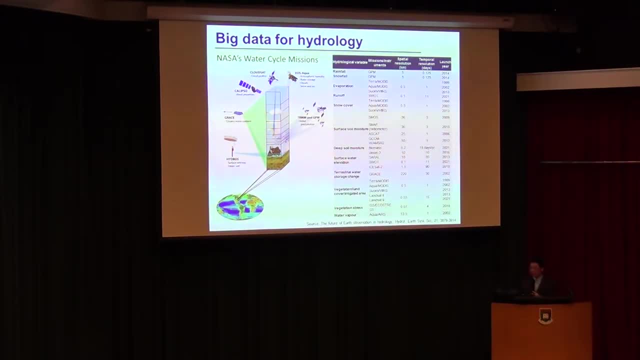 Not only for hydrological variables. Some satellites can also provide Land use information, Vegetation information. So the most common data source Is MODIS And the Landsat. You may heard about that. So that's the big data. 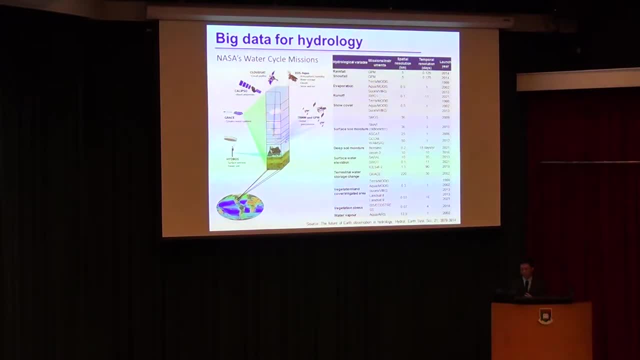 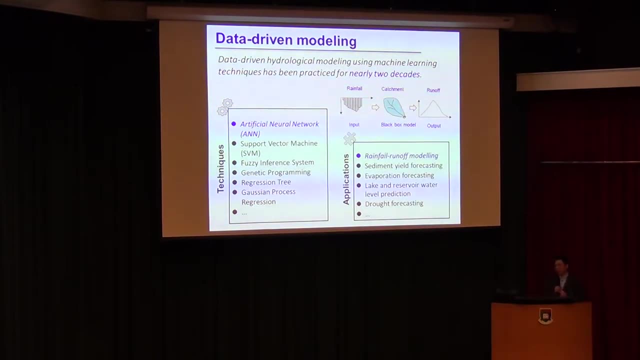 Major sources of big data For hydrology. Let's talk about data driven modeling, Because it's quite common In other fields And in our field The data driven modeling Has also been practiced. Using machine learning techniques Has also been practiced for a while. 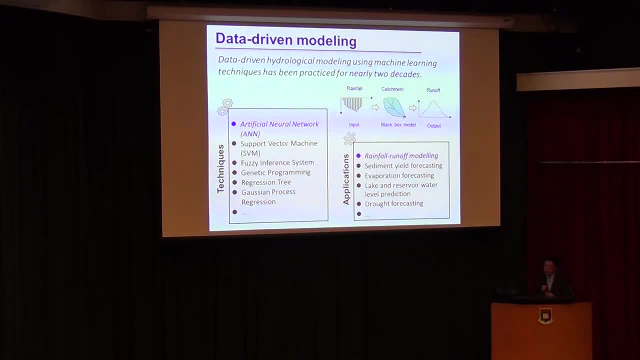 For nearly two decades already. So in our field The most frequently used approach Is just ANN, The classic ANN, Artificial Neural Network, And also like a support Macto machine, SVM Or genetic programming. Yeah, We have many applications of them. 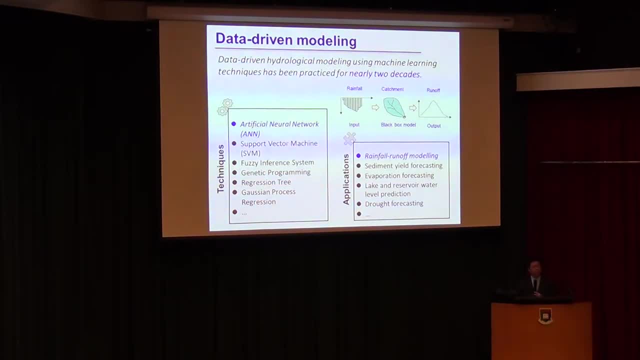 And the most classic problems Addressed by data driven modeling Is a rainfall runoff model, That's, If we know how much precipitation, We would like to know How much would the flow be. So that would be important For water supply. 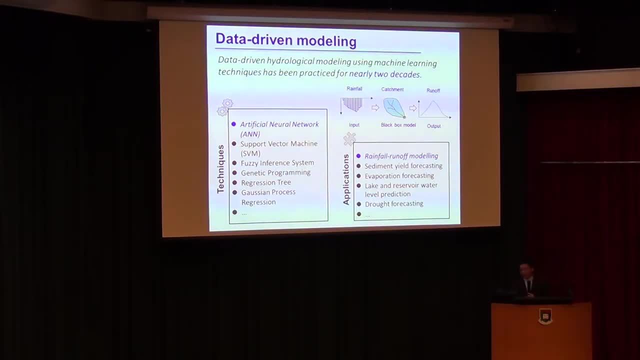 And all, And flood control, Okay. So yeah, Although there are many applications Of data driven models, So it's still not Considered the mainstream In the hydrological modeling By our society. So the main problem is: 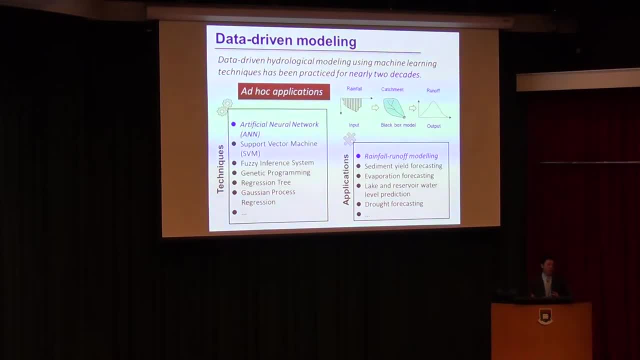 All those applications Are mainly ad hoc applications. It's very difficult to generalize These data driven modeling studies. Okay, So this is the background. Then I will move to Three study cases My group has Has done Okay. 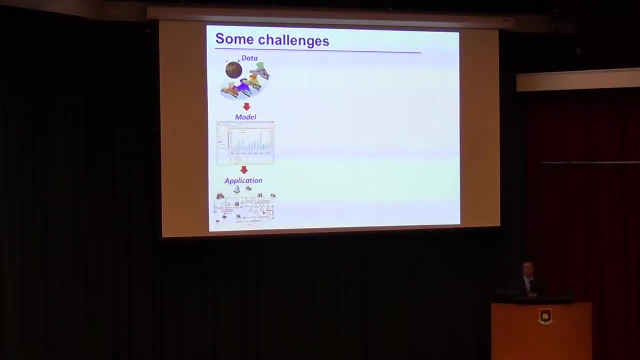 So before going to the Cases, I would like to Say something about the challenges here. So I put data model applications, The chain, here, And for each node of the chain I would like to Discuss the Challenges. 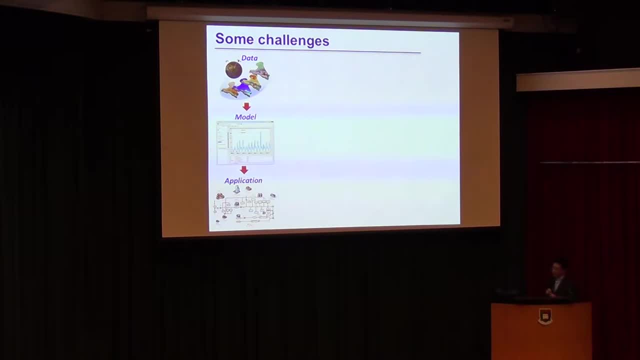 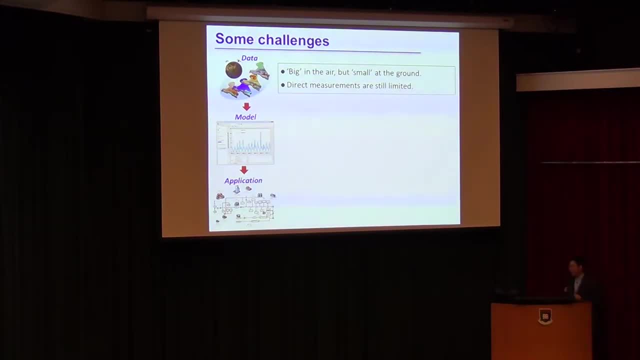 But Small At the ground, Which means We- It's a big data Really, Mainly from the Satellite data, But at our ground We really Lack of high frequency, Large volume Observational data And 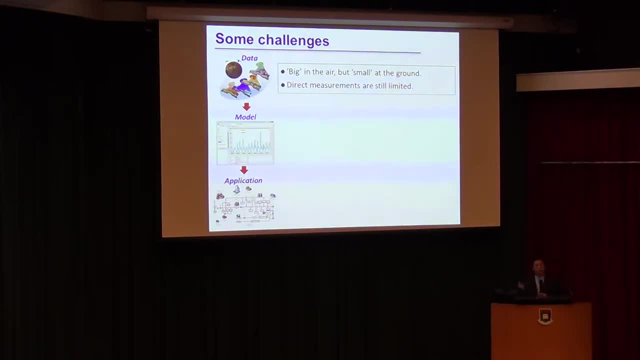 The second one Is We are still lack of Direct measurements Because The radar Or the calibrate their data against some ground level measurements but the groundwater measurements are still very limited because those devices are expensive and also those devices only provide you. 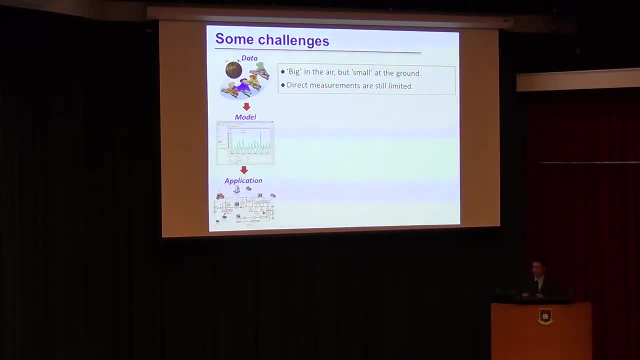 point measurements, not aerial measurements. so that's two big challenges for the model on the once. on one side, the physically based models involve significant uncertainty. so in past, like 10 years, most of my work address the modeling uncertainties of physically based model. i think that's why i was invited, because i published a series of paper about modeling. 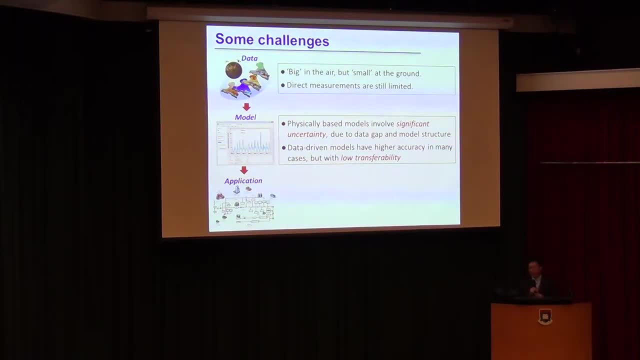 uncertainty. so the uncertainty actually came from the data gap and the model structure. so on the other side, the data-driven models have higher accuracy in many cases. so that's proved by many applications. so the data-driven model can provide you better predictions, especially those short-term predictions. but the problem is they have 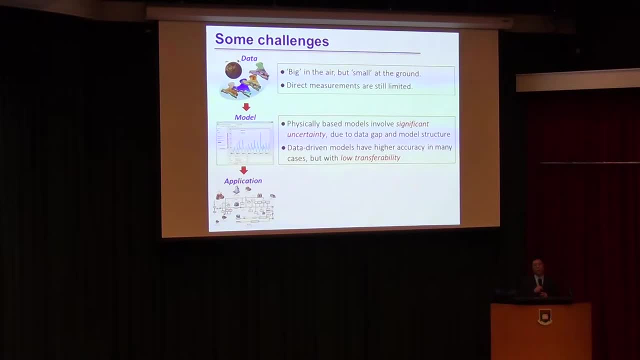 very low transferability. it works for one area but it doesn't work for another. at the application level, one problem i would like to point out is that physically based model can offer deep insights, but they are very computationally expensive. okay, so, although we have the ability to use the data-driven model, to run the model, but in real world, the daily regular 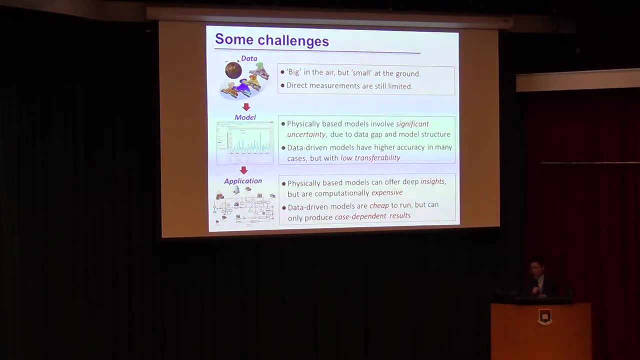 management, it's, it's. it makes no sense to use super computer to support the daily decision, okay. on the other side, data-driven models are cheap to run. once they are built, it's very cheap to run, but they can only produce case-dependent results, and so so for one application, this model works good. 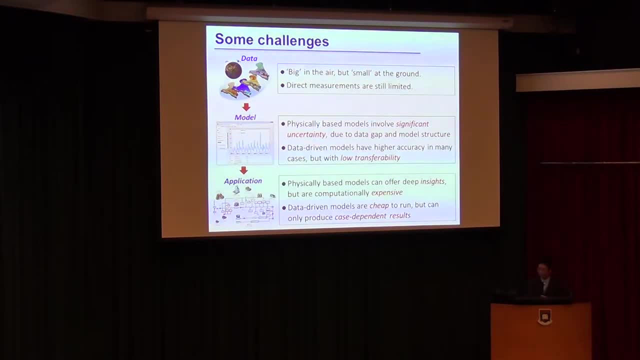 but it can't play. it's not very bad for another application, okay. so challenges means research opportunities. so i put three key questions here. so at the data level, i think a question is what kind of roles could opportunistic sensing and the crowdsourcing play in hydrologic modeling? at the model level, we need to answer this question: what kind of rows could 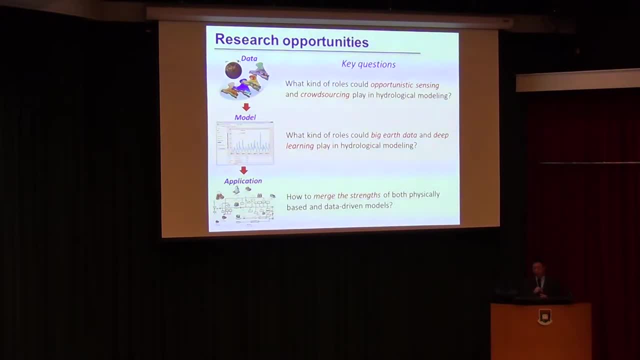 and deep learning play in hydrological modeling. And at the application level we need to consider how to merge the strengths of both physically based and data-driven models. So in the recent two or three years my research interest has shifted from modeling uncertainty into these questions. So 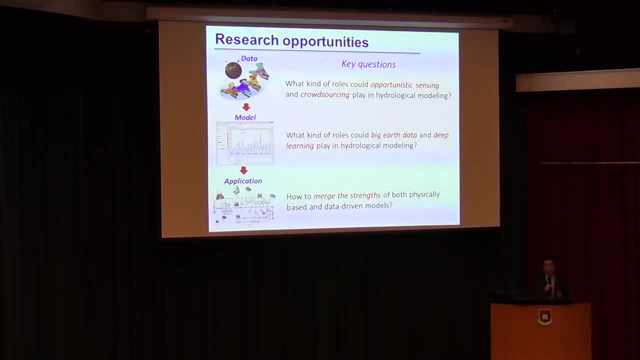 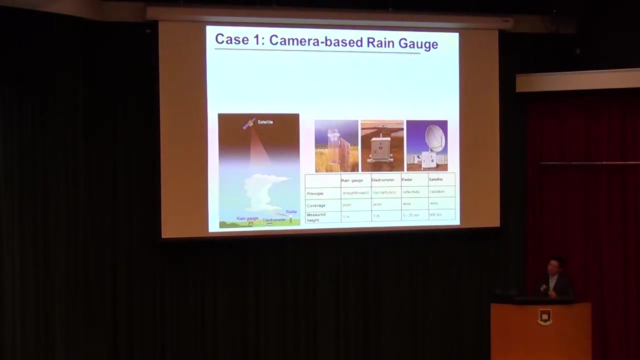 I will not do some research, it by the very preliminary. So next I will just present some preliminary research results to you and hope-, hopefully, can get some feedbacks from you. So the first case is we do a camera based rain gauge. so range of measurement Okay. so these figures show you the existing 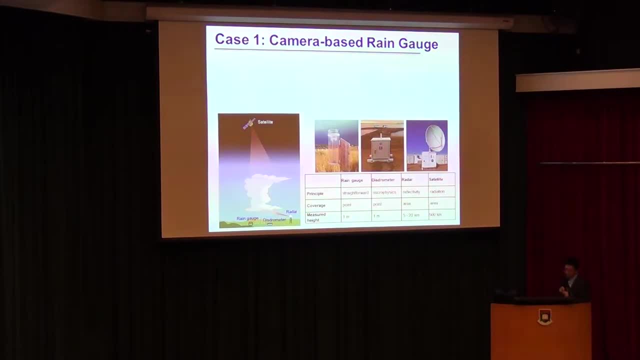 measures to gather rain data. So first they'll settlement, as I said, satellite. So satellite is based on radiation signals And it provides aerial data at the scale of this much like hundreds of kilometers. And the next one is radar Radar also gets data from the remote. 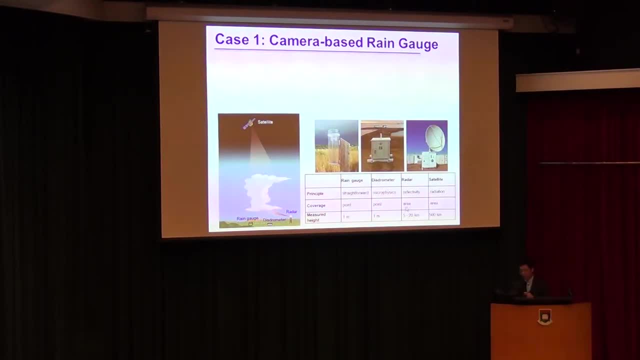 But radar depends on reflexivity. It provides also aerial estimate of the precipitation and its spatial scale is about several to tens of kilometers. Some more traditional measurement gauges. it's a rain gauge like this: It's just count how much water can be collected. 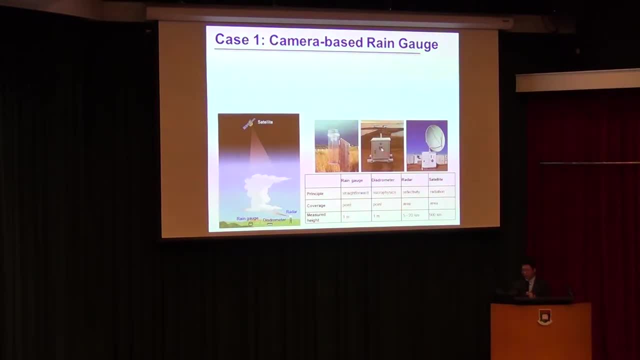 by the vessel. okay, And this one is more advanced point measurement. It's a distrometer, It's just a count: the size, the size distribution and the number of the rain drops. okay, So these are, I will say, direct measurements. 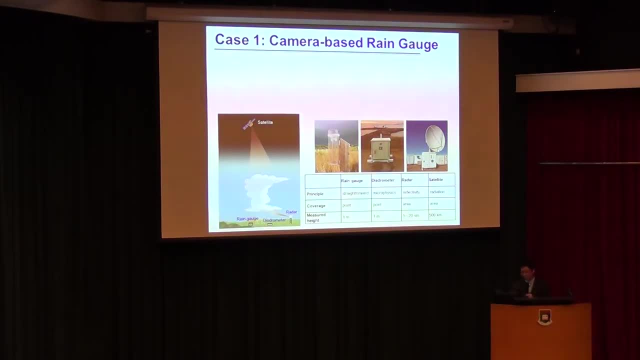 And the radar and the satellite are both indirect measurements, So these are the most often used technologies to get rainfall data. But, as you can see, so for this matter, some are just low resolution, Some are just very high cost, Some are just indirect. 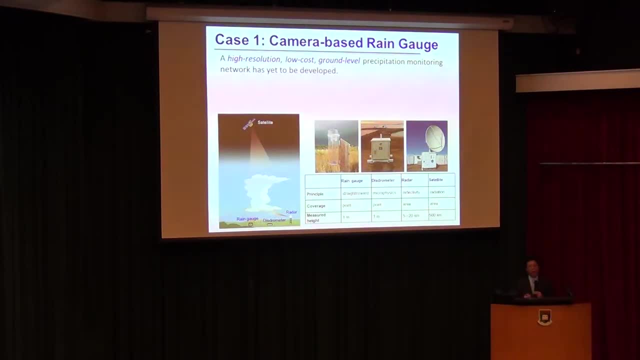 So eventually we are still looking for a high resolution, low cost ground level precipitation monitoring network. So we need such a network to really get some big data at the ground level. So in this study our idea is we just think about this question. 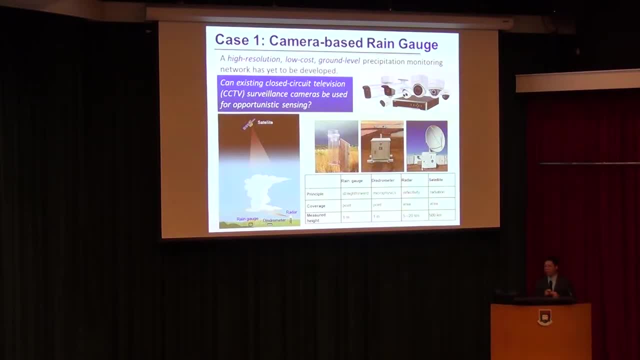 So can existing closed circuit televisions as CCTV surveillance cameras be used for opportunistic sensing? So we know there are many this kind of cameras, many everywhere. So yeah, except private space. So, but yeah, But can we use that to measure rainfall? okay, 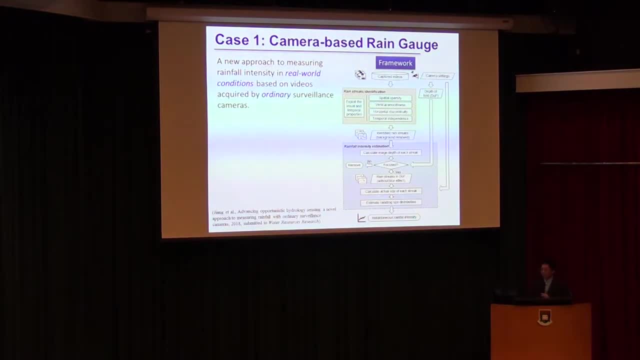 That's an interesting question. So start from this question. we developed a new approach to measure try. we tried to measure the rainfall intensity in real-world condition based on videos acquired by ordinary surveillance cameras, which means cheap cameras, not professional level cameras, okay. 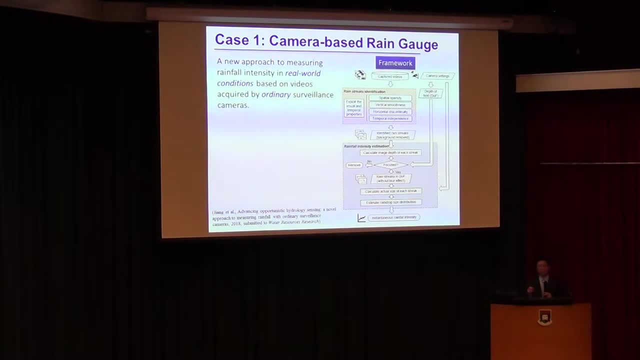 And in real-world condition, because a few studies attempted this kind of things but they just use very, very hypothesized background to do the interpretation. But we want to check if we can do that in a real-world environment and use very cheap device. okay. 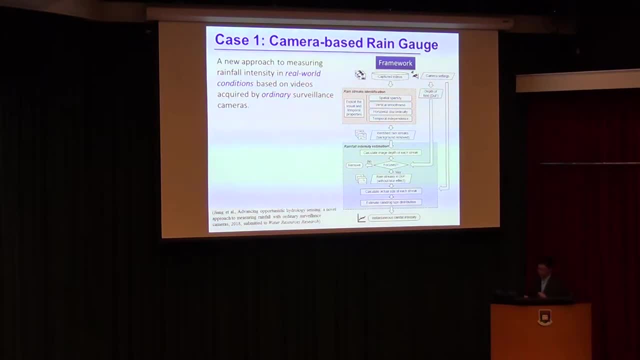 So this, the figure on the right, shows the basic framework of our approach. So it was short can be. it can consist of two parts. one is the algorithm to identify rain streaks from the rain free background, so separate rain streaks from the rain free background. that's the. 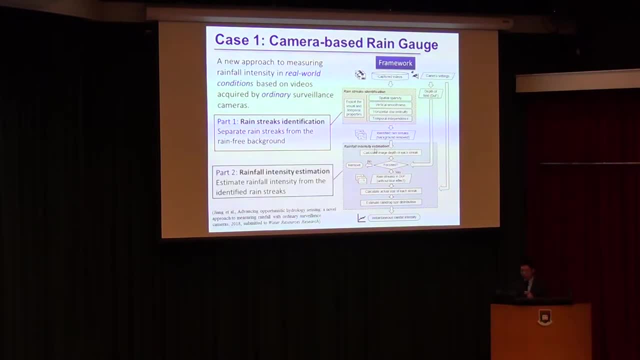 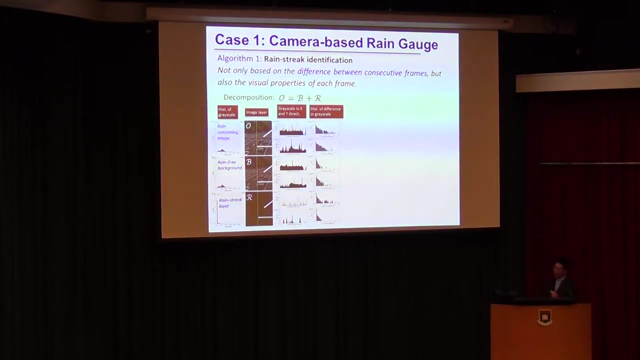 first part of the algorithm and the second part of the algorithm is to, based on the identified rain streaks, we estimate the rainfall intensity to get the the quantitative results about the rainfall intensity. okay, so this slide shows you the basic idea of the first part of algorithm. 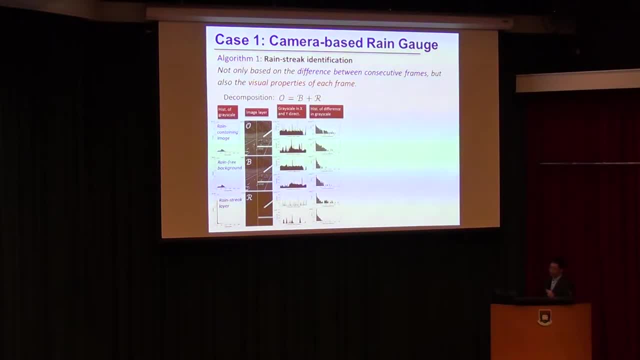 that's the rain streak, uh, rain streak identification, so, uh, so in pattern recognition, so in computer vision area. so there are many, many researchers tell you how, how to identify specific items from from a picture. but it's not straightforward to separate rain streaks from a complex image. 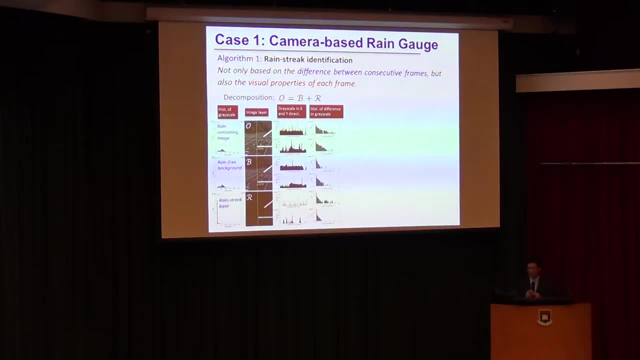 previous methods mainly address, mainly do the separation based on, mainly based on the, on the difference between consecutive frameworks. that's the algorithm, the previous algorithm. look at what's the difference between two consecutive frames, based on the difference. then it tried to separate the rain streaks. but in our approach, 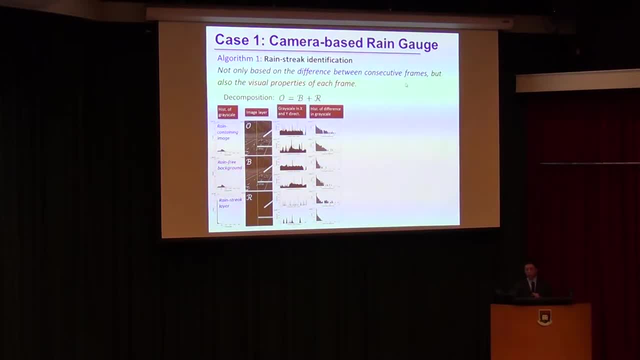 besides this, this difference, we also, the the new approach, also look at the visual properties of each frame. so it's considered more factors to to separate the the rain streaks. so, in short, so the image o can be decomposed into the background, image b and the rain streak, rain streak layer. 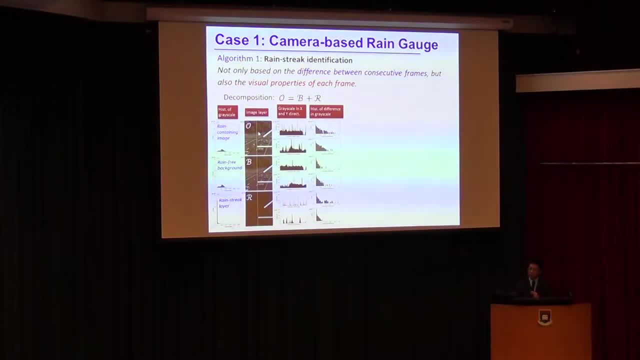 r. okay, so this picture shows you the original one, the background one and the the separated ring streaks. okay, so these two, these three is the first column and the third and fourth column- just tell you some visual properties of different layers in this frame. okay, so our idea is to to come up with this convex optimization problems. 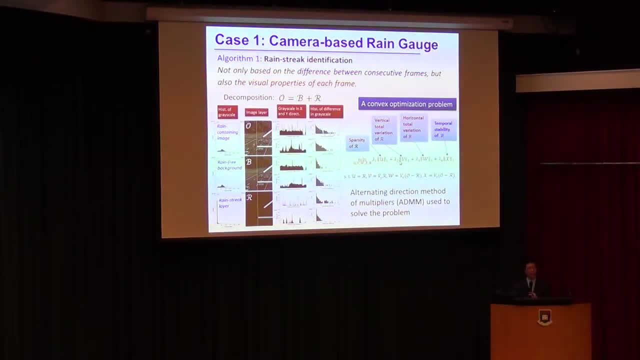 so the objective function actually consists of four items. let's look at the last item first. the last item is actually to see the. it's actually what i mentioned here. so that's the difference between consecutive frameworks. so it's represented the temporal stability of b of the, the background information, which means we want the separated background layer. 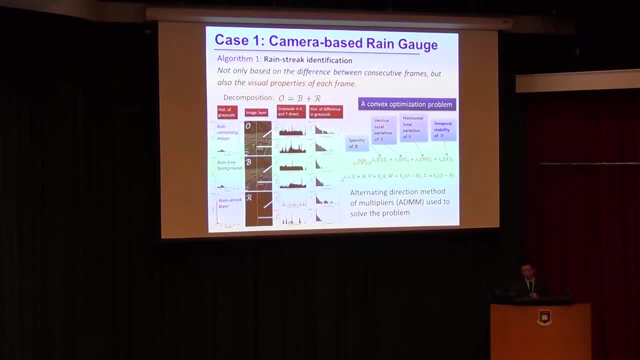 as stable as it can, because it's a minimization problem and there are three additional items. the first one is actually the, the, the sparsity of the ring streak layer. okay, that's an l1 norm of this matrix, yeah, so the idea is that we know, like this image shows, the ringstreaks are sparsely distributed in the space, so we want to. 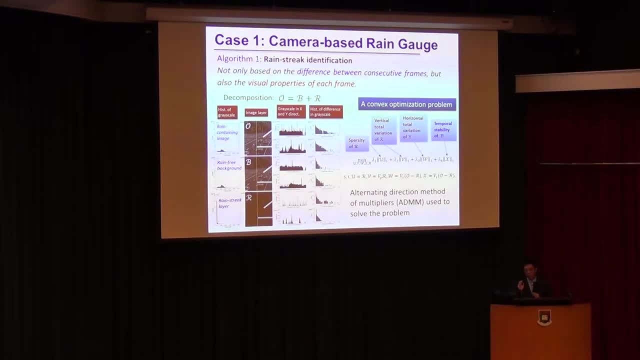 see it's uh, we, we assume uh, the ringstreaks should the the this sparsity should be, we should see sparsities from this layer and the second and the third items actually represent reflect the vertical total variation that's. the yellow lines indicate, along the yellow line, the. 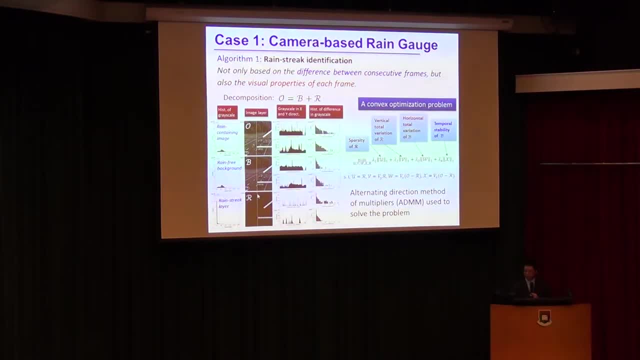 vertical one of the rainfall in this on the rainfall layer and the third one reflects the horizontal total variation the red lines indicates in B in this layer, in background layer. okay, so so this, just the idea, is that, like in the rain streak layers, we want the vertically, vertically we we prefer to. 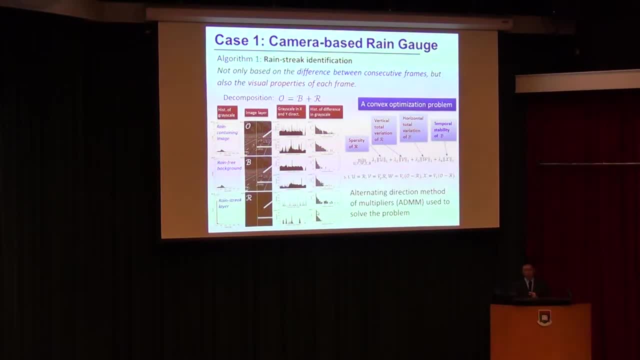 see more zero values along the zero difference along the line, along the around the vertical line. sorry, along the vertical line, because the rain streaks lines vertical lines. if there's no significant wind impact, the rain streak should be vertical lines. so we would be happy to see small vertical variations. 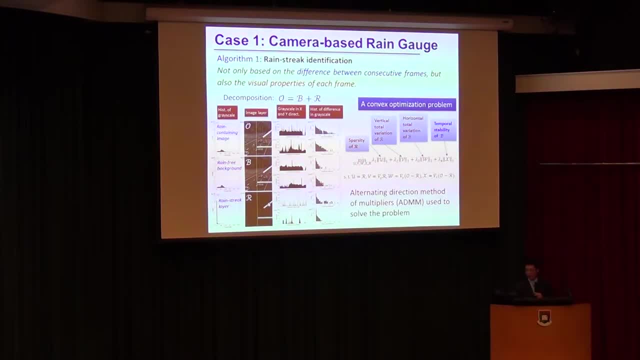 in this image, the grayscale value: small variation of great grayscale values. okay, so this is just another one to measure the horizontal change of the grayscale value in the background. okay, so this is just another one to measure the horizontal change of the ground information. so we, we did not grab this object function from the air, so 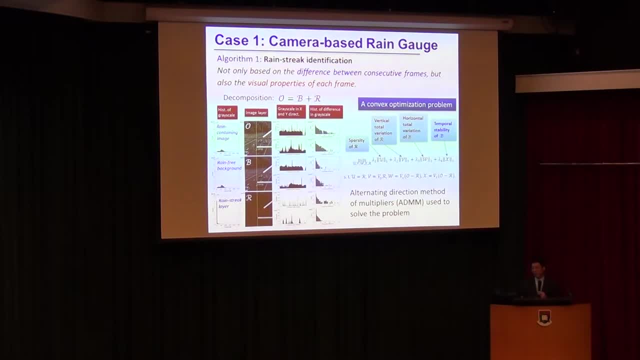 so we do not grab this object function from the air. so we actually made a lot of tests and eventually we think these four items are relevant. so to resolve this convex optimization model we use a wider use approach, alternating direction method of a multipliers, ADMM, to solve this huge convex. 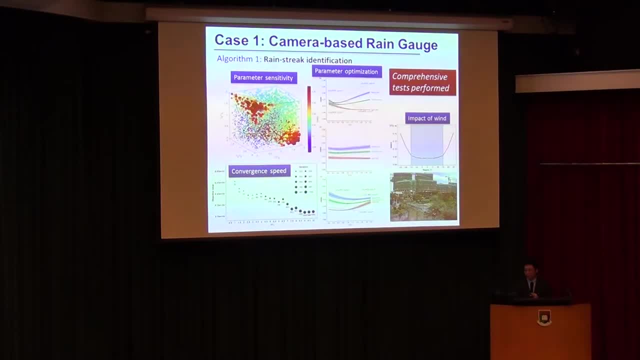 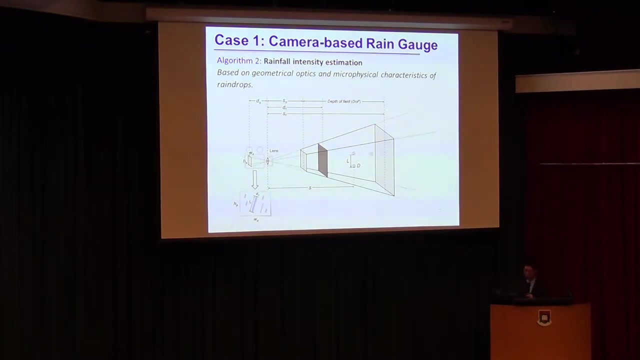 convex optimization problem. So we perform the comprehensive test to see the parameter sensitivity of the rain streak identification algorithm and to come up with some general rules to optimize the parameter choices. and we check the convergence speed and also we evaluate the impact of wind. So just to give you some idea of what we have done to test this approach. 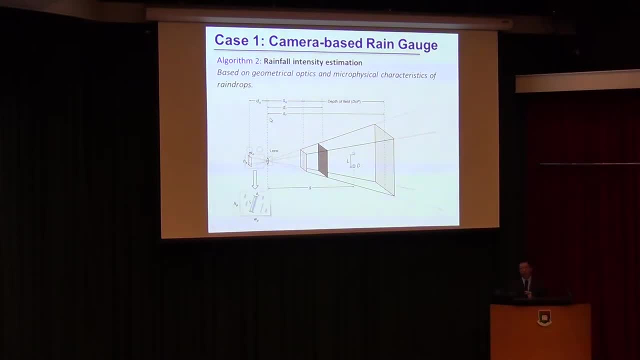 So the second part of the algorithm is to estimate the quantitatively derived rainfall intensity from the identified rain streak layer. So this algorithm is actually based on classic geometric optics and the micro-physical characteristics. I will skip all the details of this algorithm because it's quite classic. 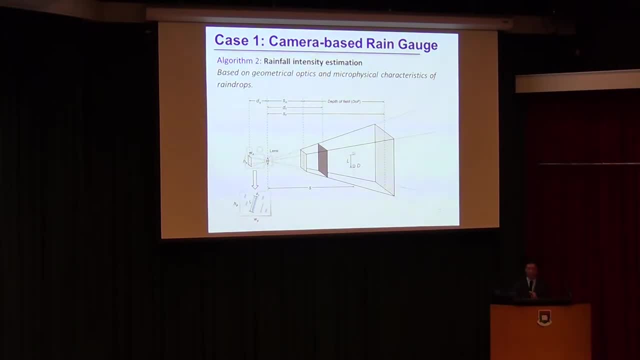 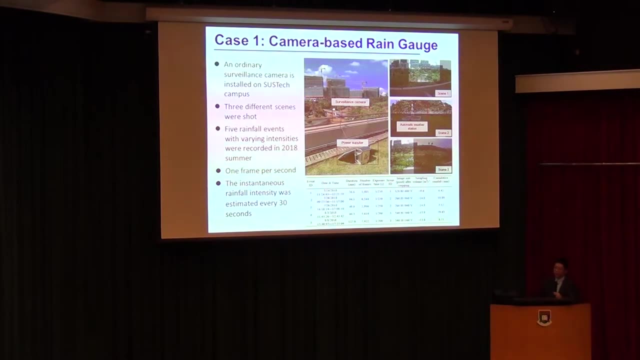 So our major innovation is the first part of the algorithm. So let's see the real-world application of our technology. So on our campus we installed an ordinary surveillance camera. This one is just here and it can change the angles so it can shoot three different scenarios. 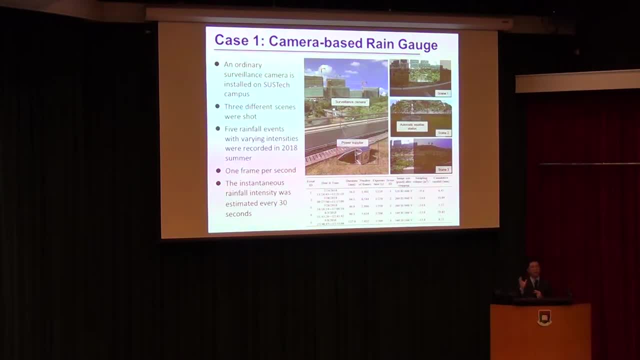 So we just check. so our method is robust for different scenes And in this summer we recorded the five rainfall events with varying intensities, and it's more than 20.. It's about six hours long video and we set the camera to take just one frame per second. 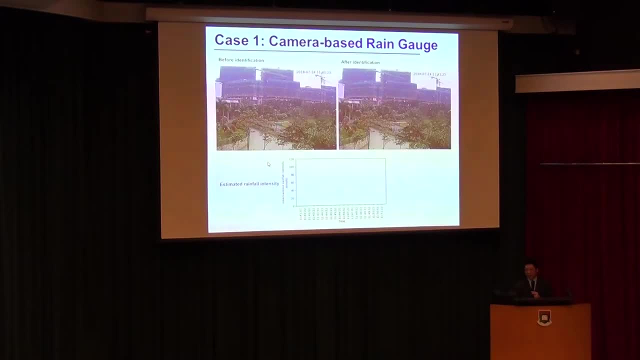 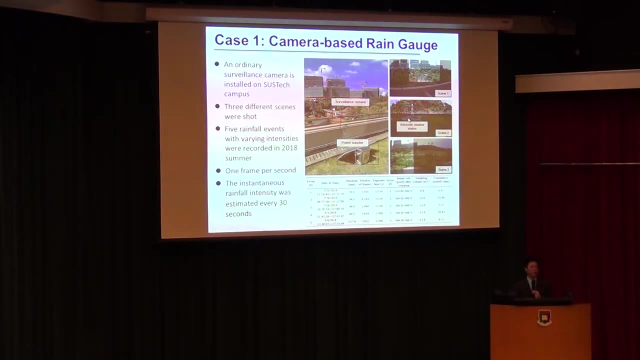 It's a slow rate and also we have this one. This is automated weather station. We need to calibrate and validate our algorithm, So we need direct measurements of the rainfall, So we also have a rainfall station. So this rainfall station measures the instantaneous rainfall intensity every 30 seconds. 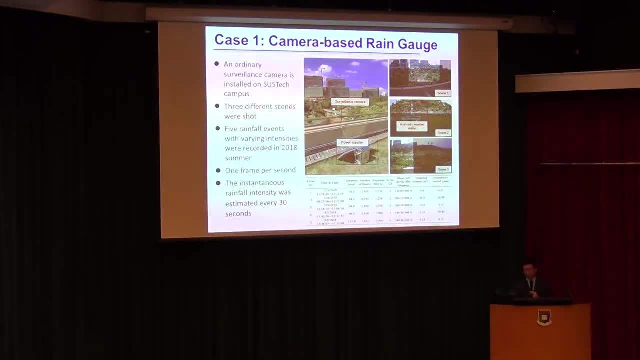 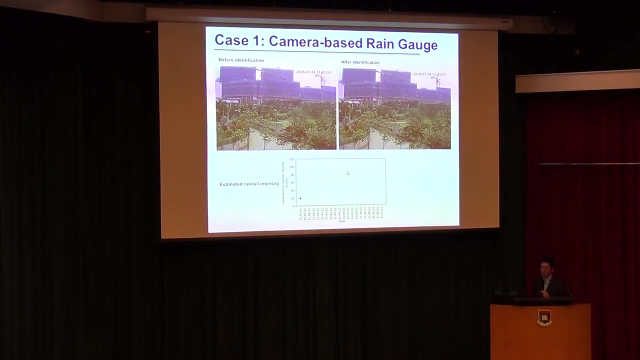 Oh sorry, every 50 minutes, But our calculation, based on our computer vision, our calculation is 30 seconds every 30 seconds, But this measures every 15 minutes The cumulative rainfall in every 15 minutes. So this video just give you an idea of what this method can do. 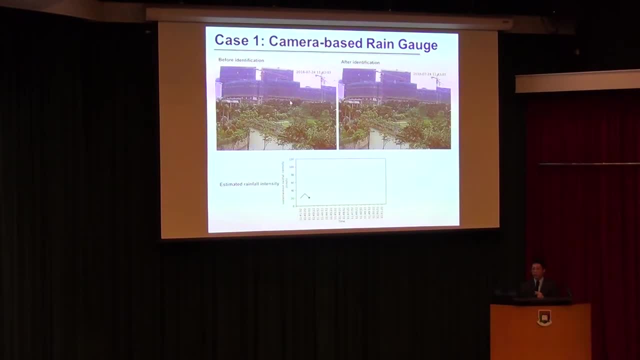 So the video on the left tells you the original video of the rainfall And on the right the video after identification. As you can see, the red Dots, red shapes, represent the rain streaks identified by our algorithm. So with this technique, we can. this is the rainfall intensity derived from the video. 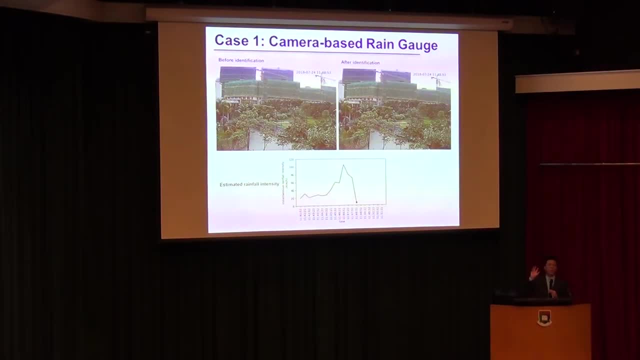 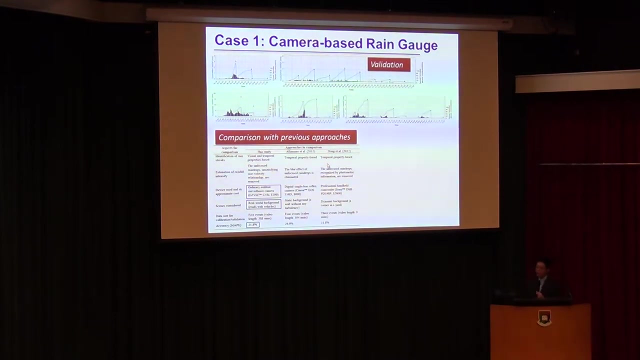 So it basically tells you, once we set the camera there and we can give you real time Data about the rainfall intensity. So how good is the result? So we this. these five figures tell you the validation results. So the red dots represent the accumulated rainfall volume, measured every 15 minutes by the rainfall station. 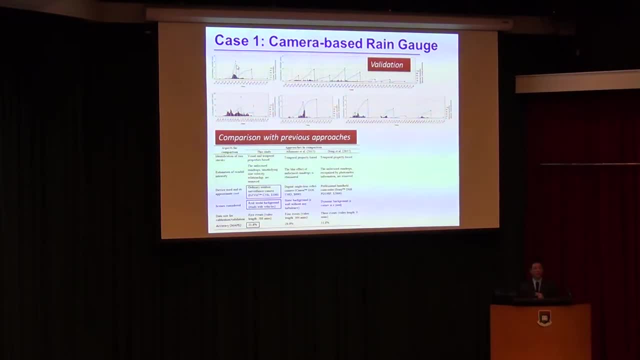 And the blue line tells the trajectory And the blue line tells the duration of our estimation. So we just compare the blue line with the red dots. As we can see, our algorithm generate very good results. But in certain cases, like this one, 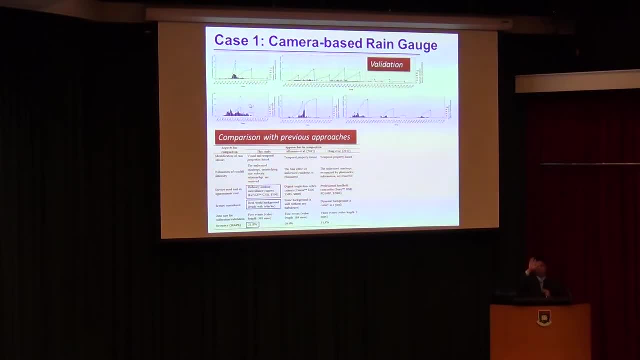 So this is a really huge storm When the storm is very huge. So it's just blurred And the performance of the algorithm is not that good, So it means we still need to improve it to deal with very huge storms. Okay, We before our approach. we only see two studies similar to our idea. 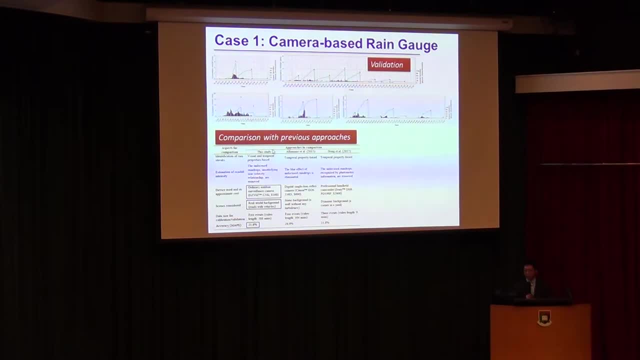 So we compare our results with previous approach. So we can see the main methods of our approach that we very cheap, We only $100. But they use professional level cameras And we consider real world backgrounds. They consider very simple backgrounds. 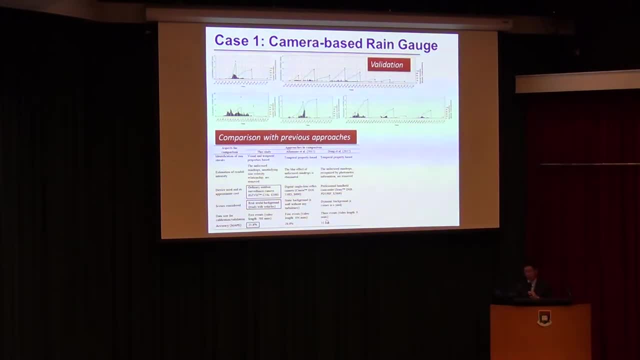 And our accuracy is also good, Better than previous study. So, in summary, low cost, more realistic scenes and higher estimate accuracy of our approach. And this study shows the great potential of using existing CCTV networks for the opportunistic hydrological sensing. 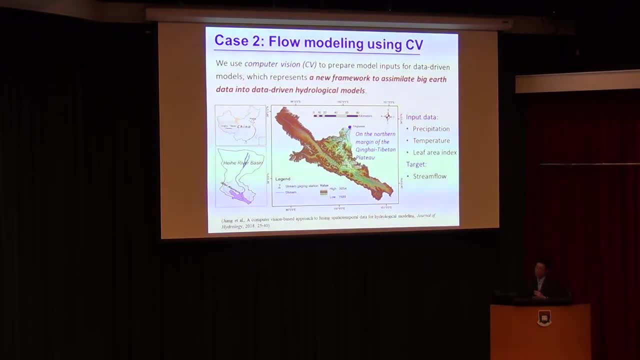 Okay, So let me talk about the case two, The flow modeling using computer vision. Okay, So, in this study, the idea is to use computer vision to prepare model inputs for data-driven models, which represents a new framework to assimilate Big Earth data into data-driven. 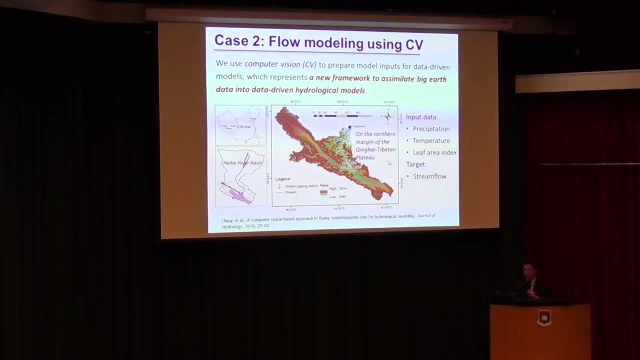 hydrological model. So we use a watershed on the northern margin of the Qinghai-Tibet Plateau as the study case, And in this modeling case, we consider precipitation temperature. Okay, Okay, So we use a watershed on the northern margin of the Qinghai-Tibet Plateau as the study case. 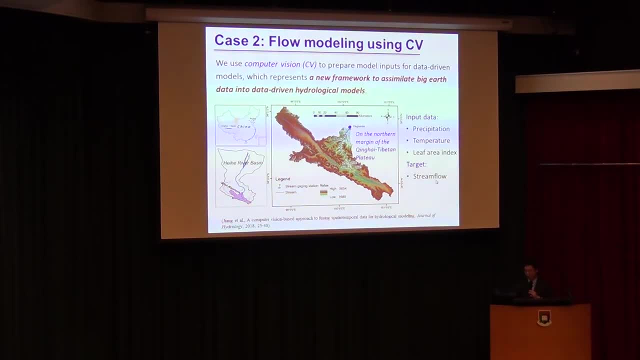 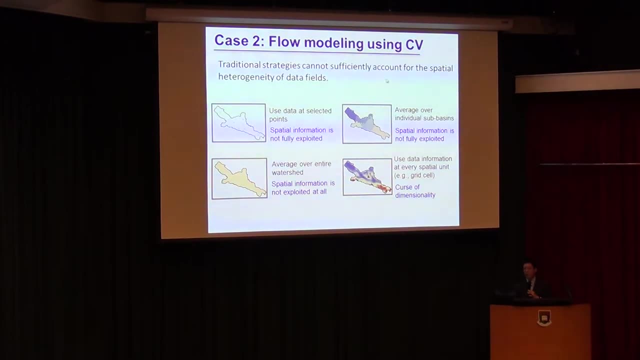 And in this modeling case we consider precipitation, temperature, leaf error index as the model input and the stream flow as model output. So what's the problem with traditional strategies? The problem is they cannot sufficiently account for the spatial heterogeneity of data fields. 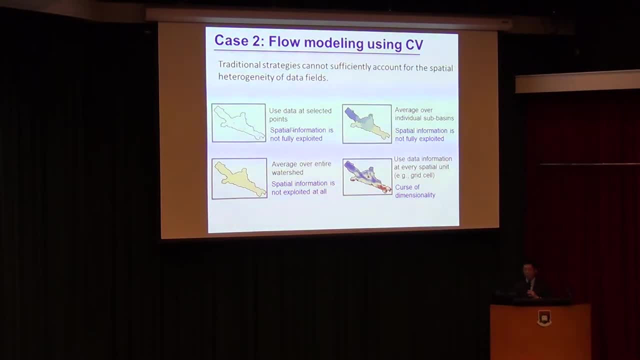 For example, in some cases people just use point some data at the selected points as the model inputs, Then the spatial information not fully explored. In other case they just average over entire watershed, Then just no spatial information is explored at all. 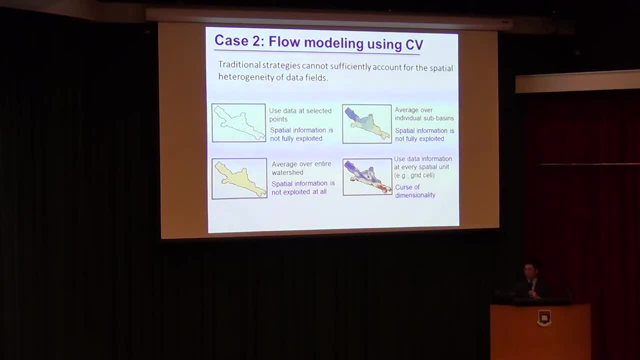 Someone tried to average over individual subbasins, like they separate a big watershed into like a tens of subbasins and average the data on the subbasin scales. but still spatial information is not fully explored. A straightforward method to account for the spatial heterogeneity is just to use data. 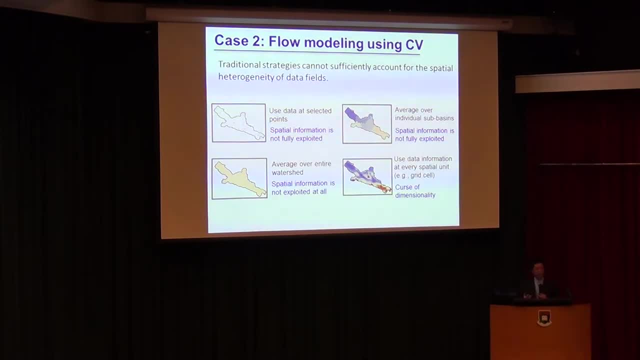 information at every spatial unit, At every grid cell. So that's the most straightforward one. But if we do this, then we will encounter the curse of dimensionality, the huge dimension of the input data. So we want to avoid this and we also want to make better use of the input data. 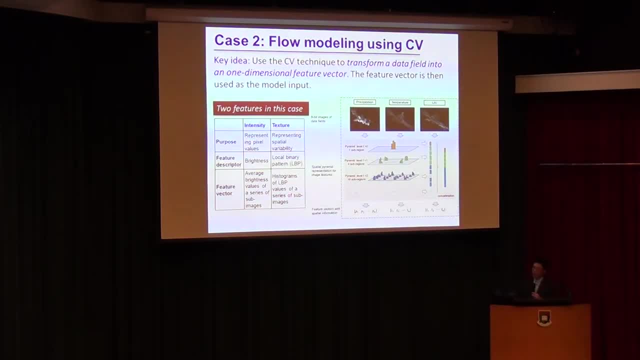 So the key idea is to use the computer vision techniques to transform a data field into a one-dimensional feature vector. Then the feature vector can be input into the data-driven model. So in our study case we can do this. We consider two categories of feature. 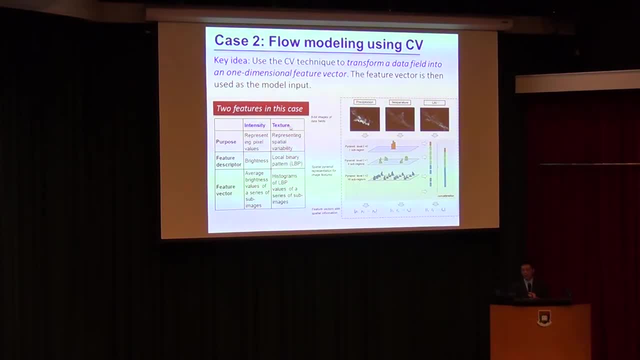 One is the intensity of the image, The other is the texture of the image. So this figure gives you the basic idea. So we have images or videos and we use computer vision technology to extract these two features using certain algorithms and we make a long one-dimensional feature vector to create such 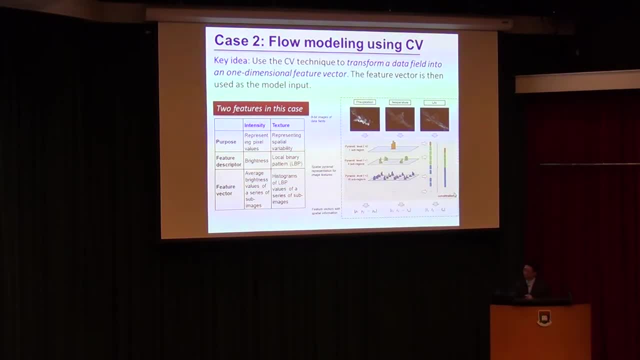 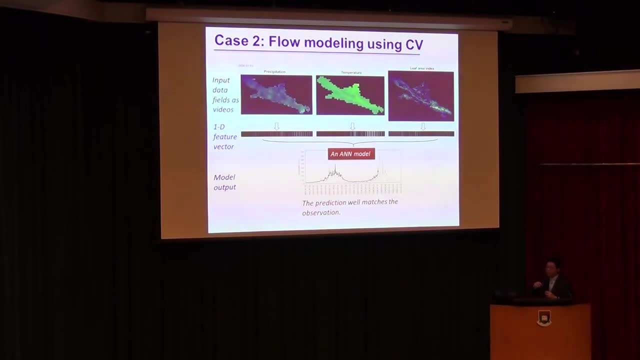 a feature vector. With this feature vector then we can do the modeling very easily. So here we see. the first row shows you the input data fields as videos. So the precipitation, temperature and the leaf air, these are all changing. Then the other algorithm can extract and can transfer all these videos into one-dimensional. 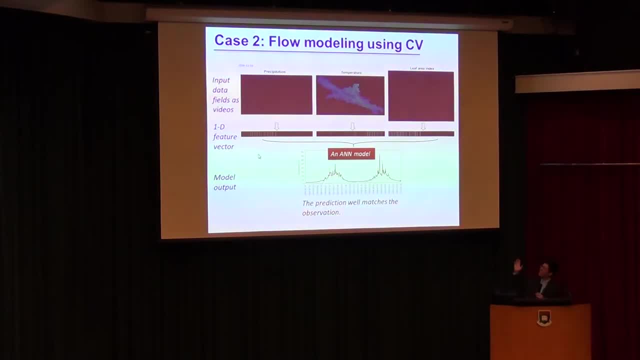 feature vector which is also dynamic. As you can see, the color is changing. Okay, Okay, So this feature vector is input into an artificial neural network model and makes the prediction, as this figure shows. Okay, So this video just tells you the whole process of how to use the computer vision-based approach. 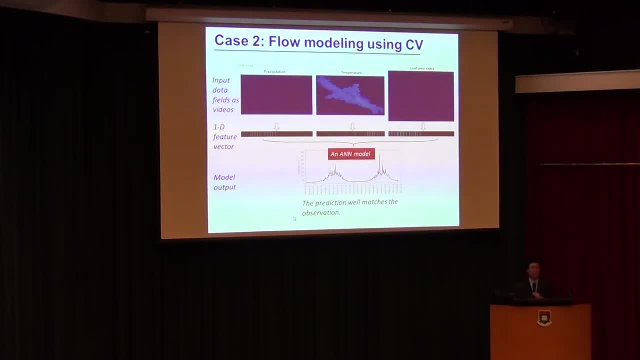 to do the data-driven model, which is quite different from the traditional way in our community. So the prediction well matches the observation, Okay, Okay. So we compare our approach with the more traditional ways to prepare the input data, So, as we can see. so the X direction shows the lead time. 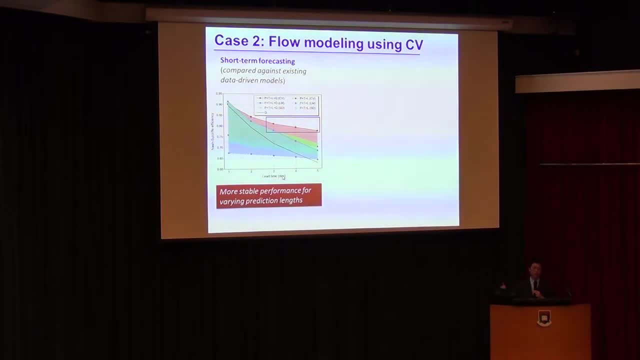 The prediction length is how many days you want to predict before word. Okay, So as we can see, so when the prediction length increase the performance, the Y axis indicates the performance. So the performance decay is quite slow, Okay, So a lot of approach has a very significant performance decay. 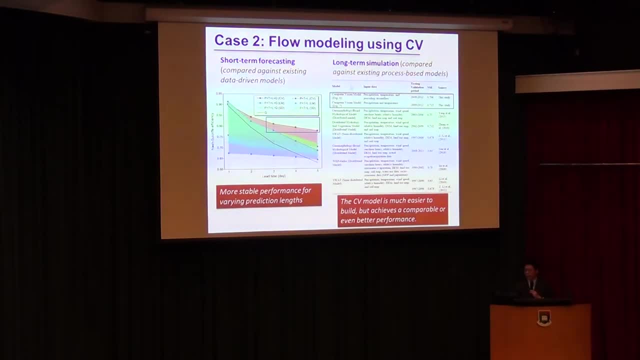 So our approach is very robust. Okay, And for long-term simulation, we compare our model with existing process-based model or physically-based model. So this column shows the model performance. So the conclusion is that the CV model is much easier to build. 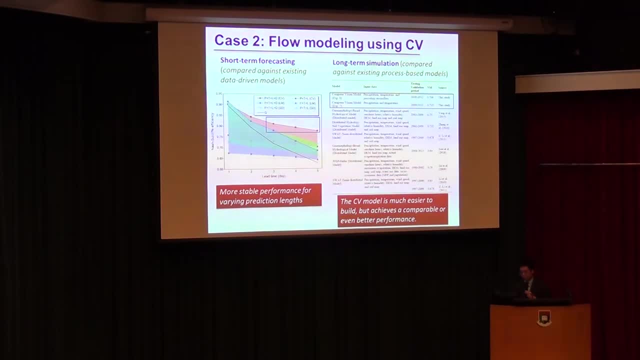 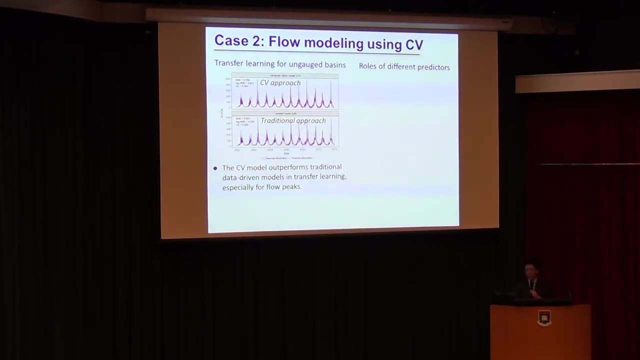 It's very easy to build but achieves a comparable or even better performance performance than those existing process-based models. So also we check the capability of transfer learning for ungauged basins, so we can see our approach works better. And also we argue that the framework we proposed gives us the flexibility to fuse multiple 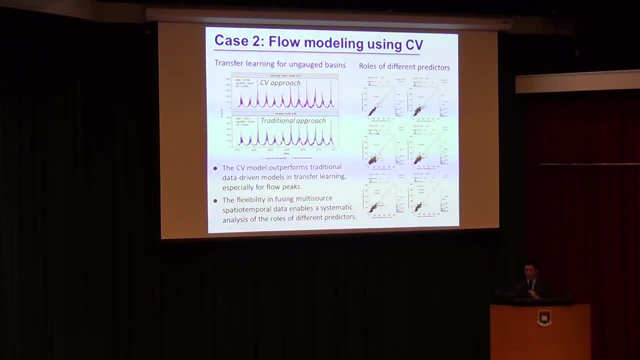 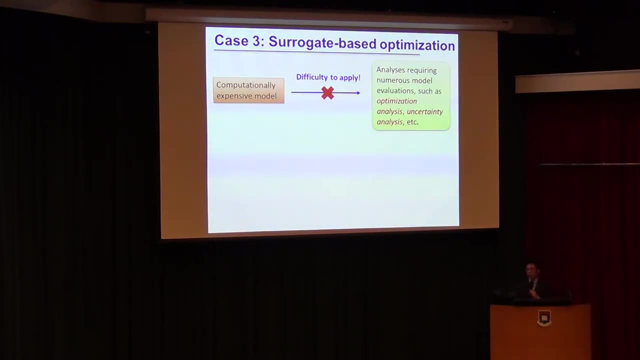 source data and assess the roles of different predictors. So the last case I will go over very briefly. so it's about the surrogate-based optimization, Because the physical-based models are very expensive, so it's very difficult to directly use them in analysis, which requires numerous model evaluations, such as optimization analysis. 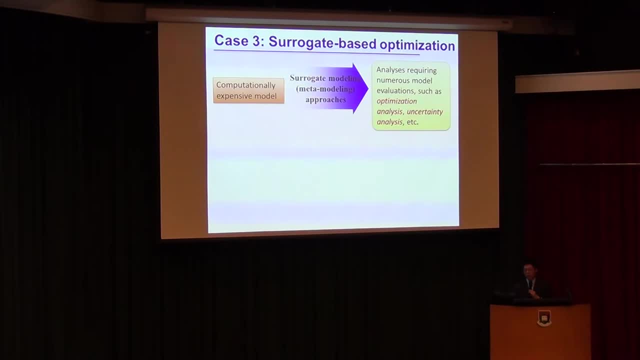 uncertainty analysis et cetera. So and strategy is just to do surrogate modeling or coordinate modeling. So surrogate model can replace the original model Fully or partially in the analysis. it's more, cheaper and it's usually in the form of responsive surface. 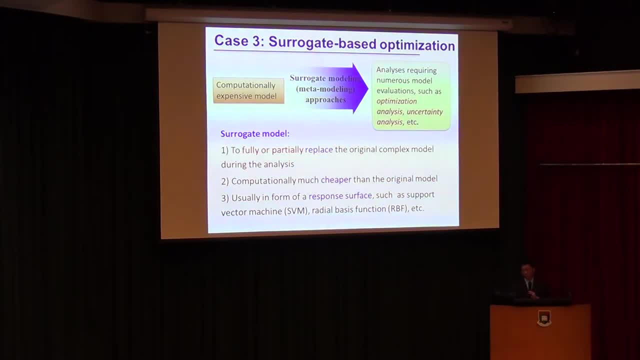 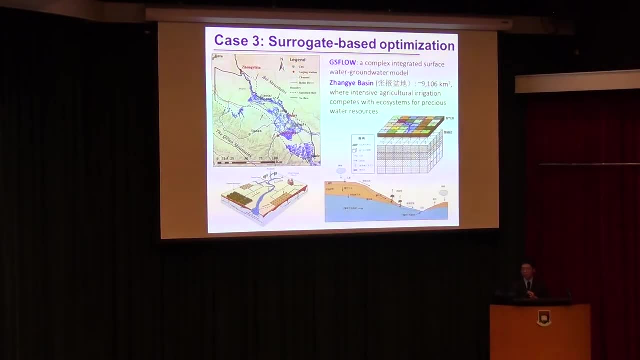 That's where the machine learning can come in. So machine learning can be a good approach to come up with some response surface. So we build a model for a watershed in the western part of China which is about more than 9,000 square kilometers large. 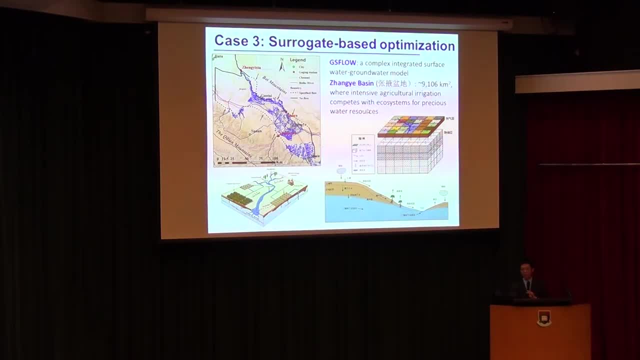 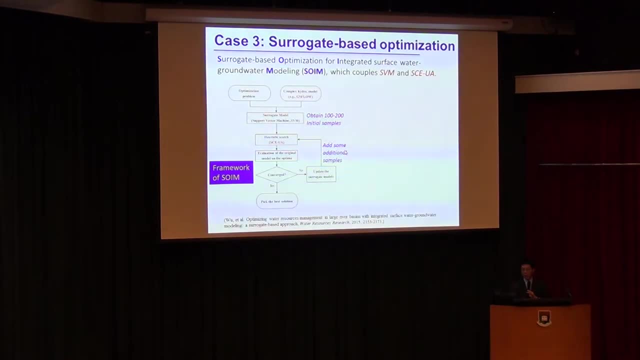 We use different kinds of agricultural irrigations, are computer with ecosystem for precious water resources. We have built a very complicated physical-based model And then we develop an algorithm. So this algorithm, this algorithm to optimize something by incorporating the physically-based model. 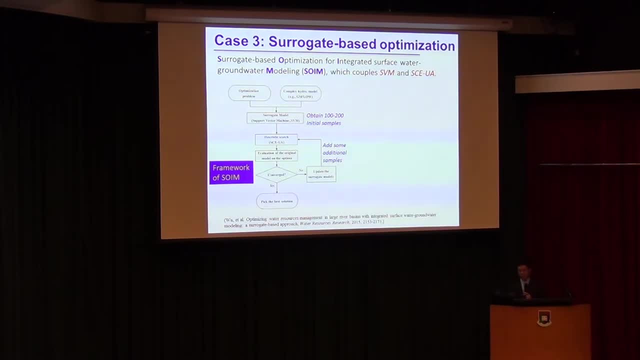 So if we use an original models that would be very computational expensive. But this algorithm, in this algorithm, If we use the original model, Would be very computationally expensive. we coupled the support vector machine with a heuristic search approach. So basically the basic idea is in the search. 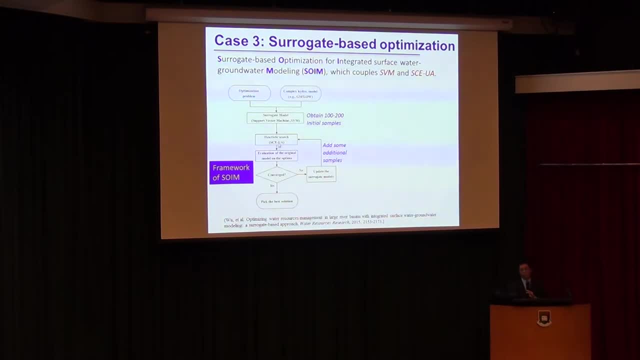 we don't have to use the original model every time. We only need to use the original model hundreds of time. Then we can finish the whole set of optimization And, for example, we use like 200 initial examples to start with and the optimization can converge. 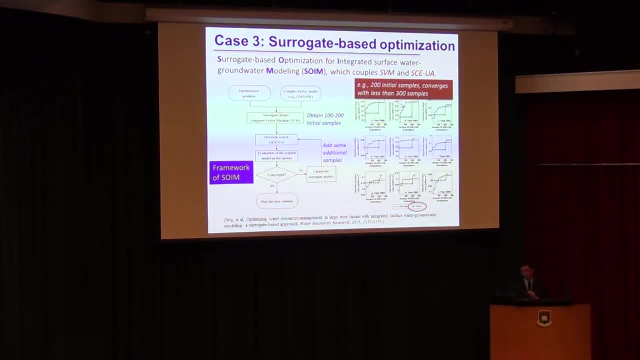 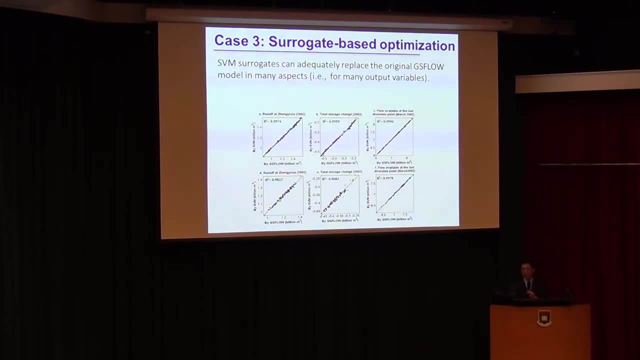 with less, within less than 300 samples. So the surrogate model based on SVM can adequately replace the original model in many aspects. So this figure just tell you it can do good job for many different hydrological variables. So it just show you that in this case, 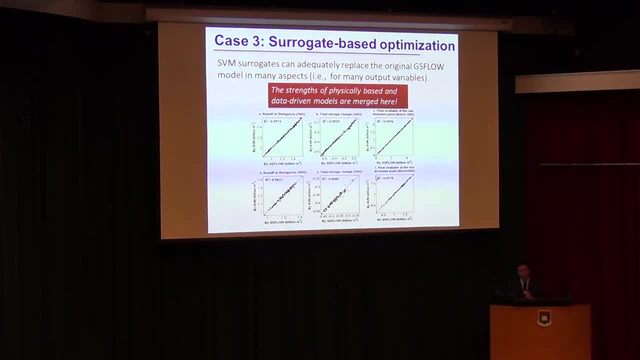 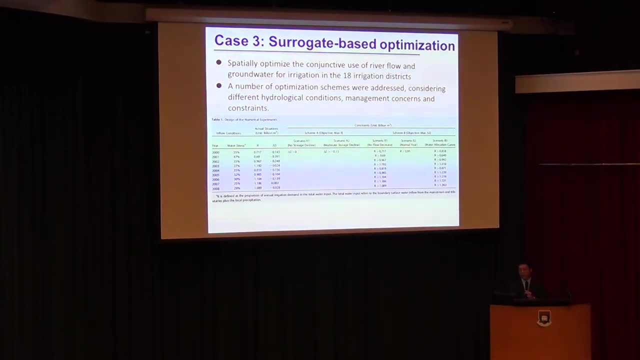 the strengths of physically-based and data-driven models are merged here, So we perform a number of optimization schemes, considering different hydrological conditions, management concerns and constraints. The main point here is, if we want to do all these optimizations, use the original model. 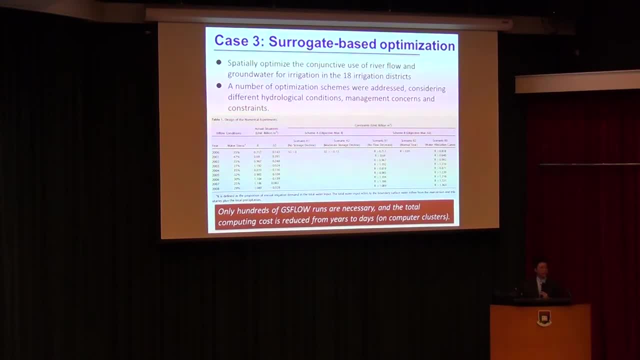 even on computer clusters. we need years to finish that, But with this surrogate-based model to use the machine learning to replace the original model, so we can reduce the cost from years to days. And here just an example of the optimization results. 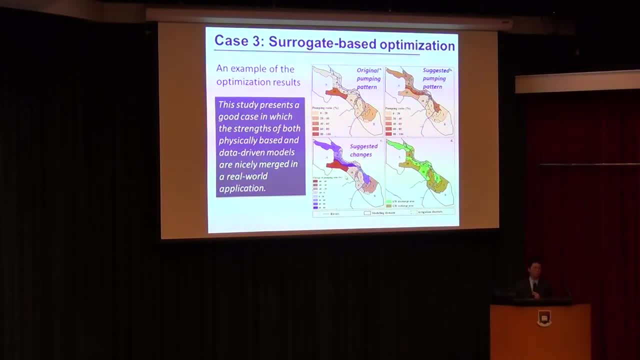 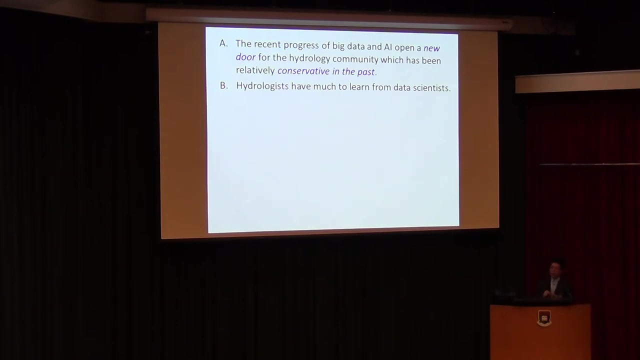 So it's tell you where to pump more groundwater and where to pump less groundwater. so so in some ways, this study presents a good case in which the stresses of both physically model and they dream models are nicely merged in a real world application. okay, so finally some concluding remarks, and so the first two are: 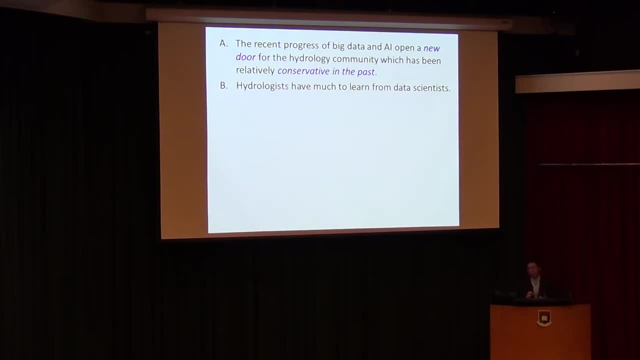 my feelings about, like these two or three years of research on big data and machine learning. so i aware, i'm aware, that the recent progress of big data and ai open a new door for the hydrologic community, which has been relatively conservative in the past. so, to be honest, our 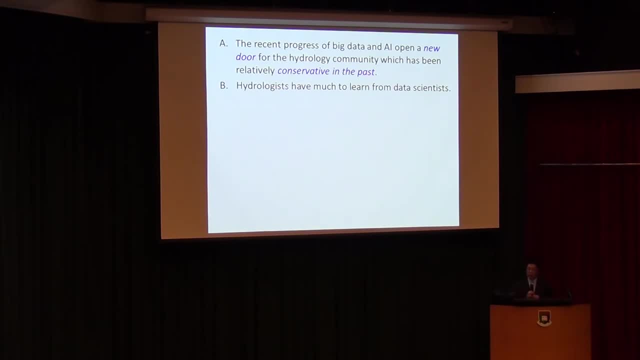 community is very conservative. and then i know hydro hydrologists have much to learn from data scientists. that's why i'm still here, although i'm nervous because i'm really out of this community. and the next three points is first: opportunistic sensing can help us all. 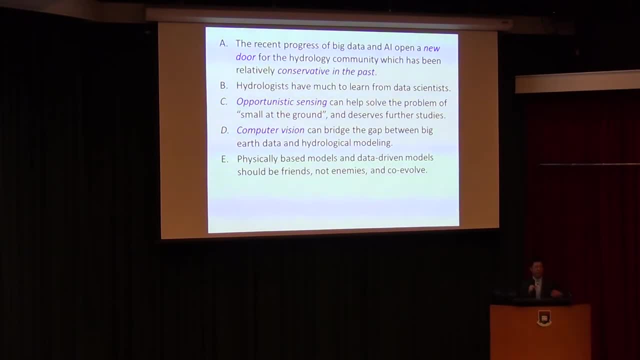 the problem of small at the ground, like the camera-based ring gauge i have shown to you and definitely deserves for the studies. then computer vision can bridge the gap between big earth data and hydrological modeling, as i showed in the second study case and, as i showed in the last study case, physical based model and daydream model. 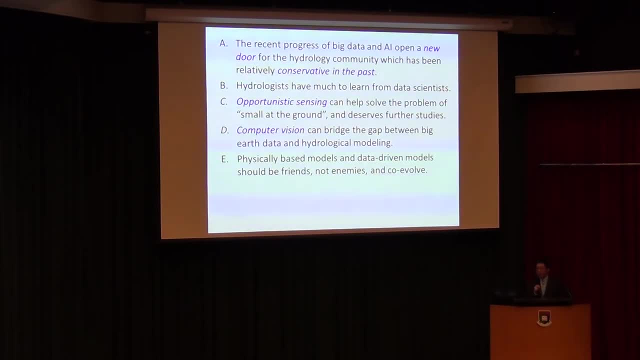 actually should be friends. they are not enemies and they they can co-evolve. because in hydrological community actually there's debate. someone thinks that daydream model using big deep learning may replace the physical based model, but others think a way to go. but i think they are not enemies. they should make friends and call you: evolve, so eventually. 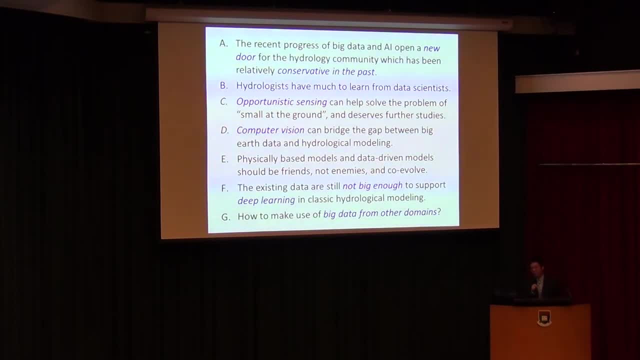 two questions. first, of the existing data are still not big enough to support deep learning. so actually, So my group- have tried different cases to use deep learning for hydrologic modeling but we have not achieved good results So I didn't present that. So not big enough for deep learning. 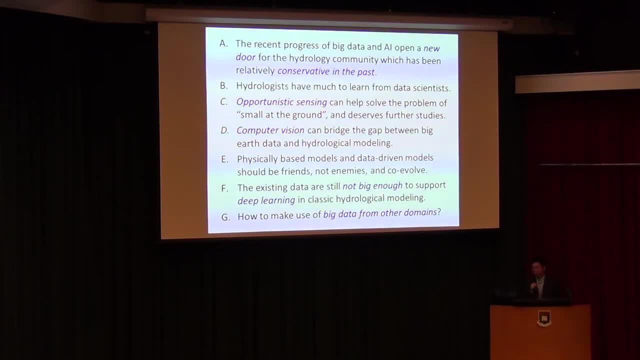 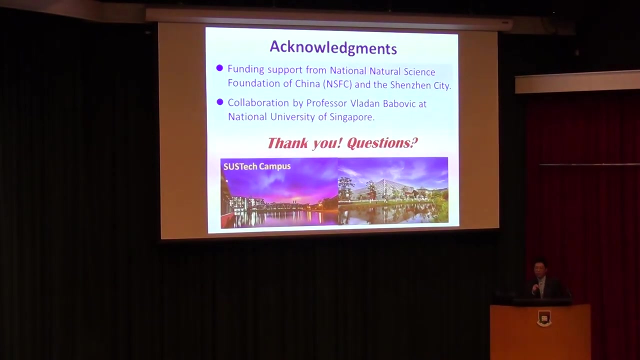 for classic hydrologic modeling. And the last question is how to make use of big data from other domains, like the internet. all sorts of socioeconomic big data is still a big question, So more research are expected. So finally, thank you for your attention. 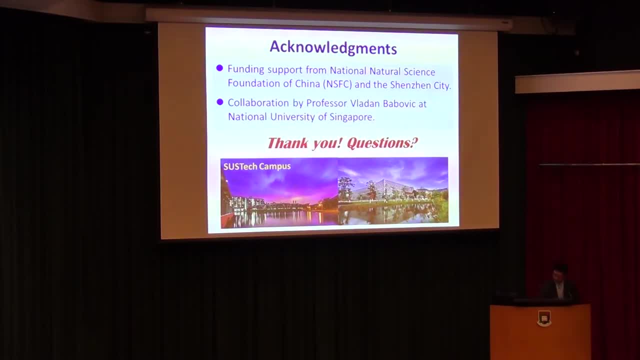 And that's all for my presentation. Thank you, Question. So I have a question. No, You have a question. OK, go ahead. So I appreciate you mentioned about the transferability. Regarding the data-driven modeling, I think this is a general question, for not only in hydrologic modeling. 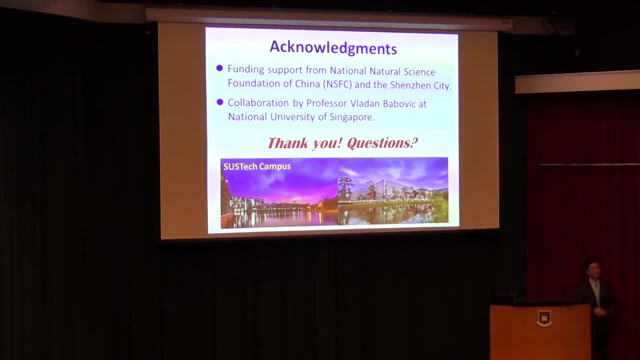 but also in many, many motor physics modeling. So in your second case, you talk about using the machine learning concept to build a model. So can you talk about the transferability issues in this case? OK, thank you for the question. So, in that case, what we have done? 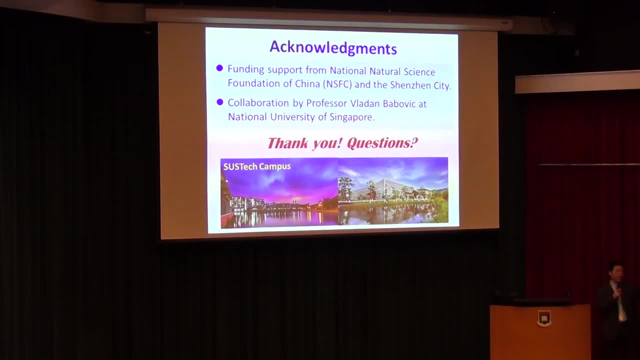 is, we calibrate the model in a part of the area And we use that model in another part of the area to see if it works. So it works in our case, because these two parts are still not far away from each other, So they still share some common features. 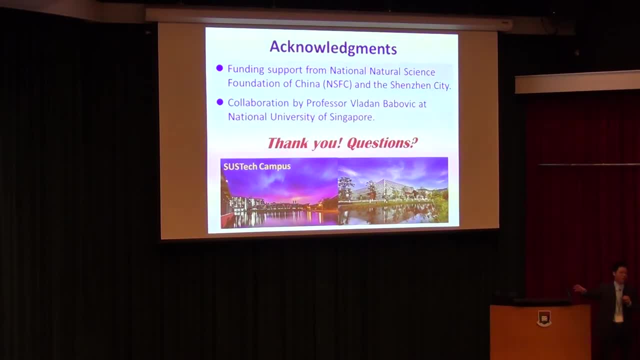 I'm not sure if I pick another faraway world that works good. I'm not sure, But I think it was not that good in that case. Yeah, So the transferable learning I have done in this study case is still very rudimental. 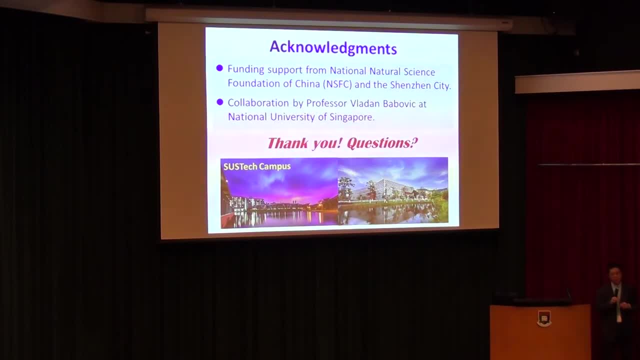 So two areas not far away from each other, It's basically just not big enough. So if we have global data sets, so we may make that general data-driven model at the global level. So it's a way to go, I think. 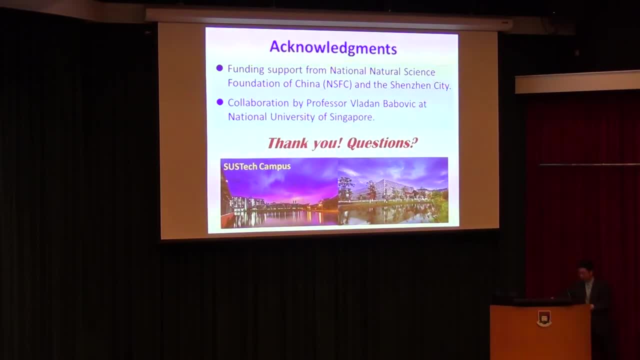 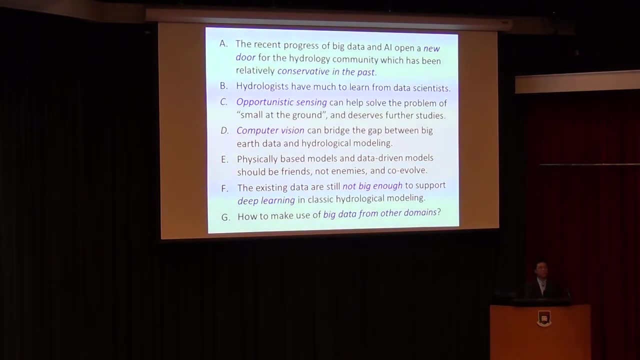 OK, Thank you. Any other questions? Can you go on the previous slide I have mostly commentary but questions. But I like some of these bullets And so you say physically-based models and data-driven models should be friends. So in many ways it's not one or the other actually.